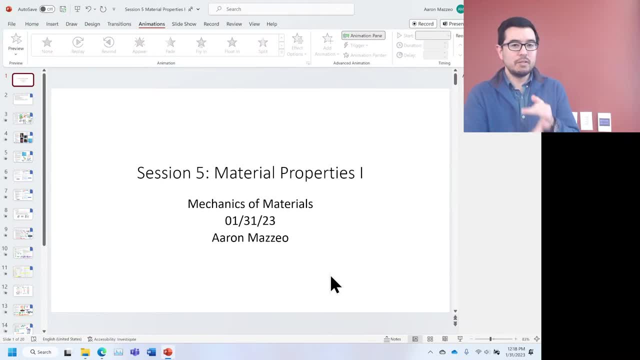 done digitally, but it needs to be handwritten for exam, one which will be on the 24th of February. Any other questions? Yes, Right, iPad notes are fine, but they need to be printed on a sheet, right And a front and back. 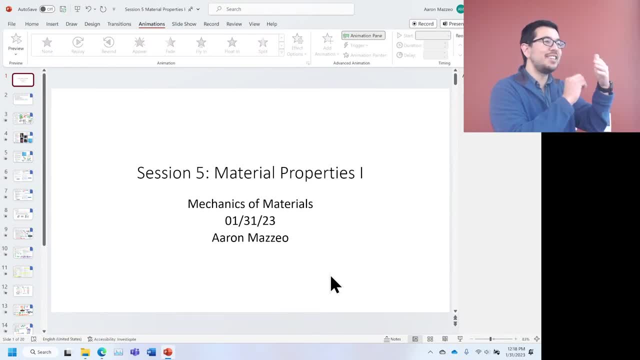 That's fine, And you know, I was a student and I did like this kind of almost micro handwriting, All right. So don't take it on the iPad and synthetically make it smaller, All right? Does that make sense? You know what I'm getting at? All right, Within reason. Okay, I don't know. I. 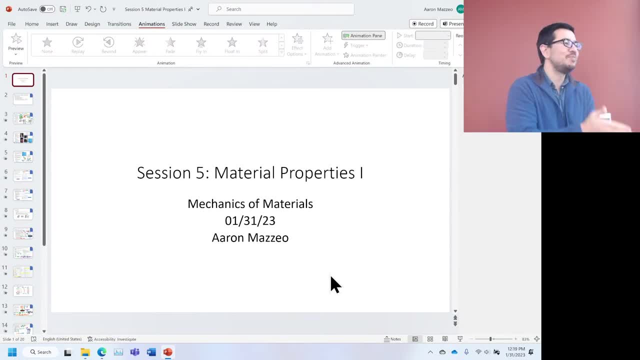 don't want to be like really, You know, I just want it to be fun. It's going to be conceptual. Okay, The exam is going to be conceptual. If you see from the past exams, it's based on being able to apply the different. 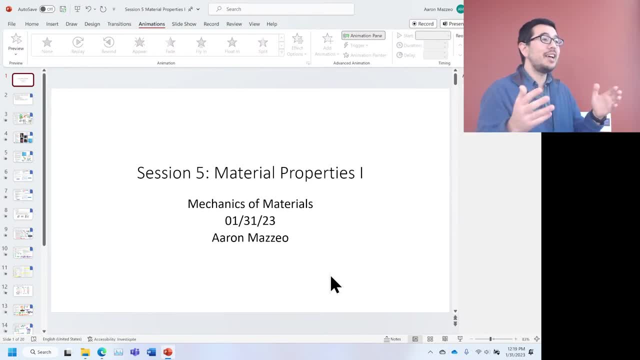 formulas. Essentially, though, you're going to have maybe 10 formulas. You write down the 10 formulas, and you know how to apply them in different orders and different ways. You're going to be- That's going to be- the name of the game. Okay, But don't randomly. 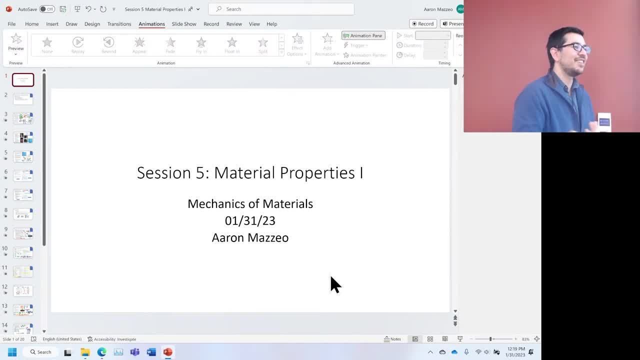 Don't randomly apply them. That doesn't go very well, of course. Okay, It's like: oh, there's a pressure, There's a force, There's- Oh, I'll just put it in this equation- You're like: no, 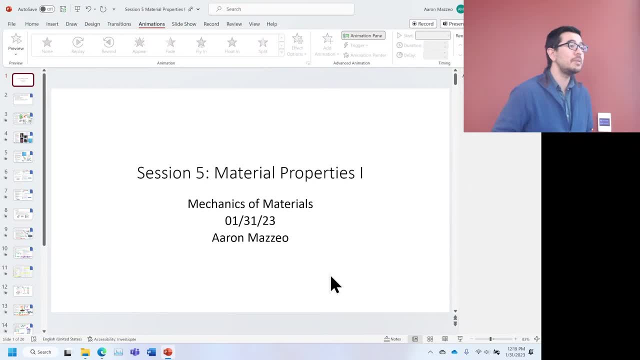 that's not the right one. Okay, I'm sorry It is. It's going to be tough. All right, It's going to be tough. So, please, please, spend some time studying. All right, It's going to be tough. 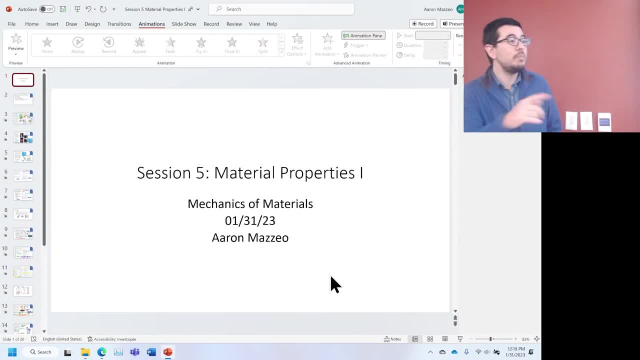 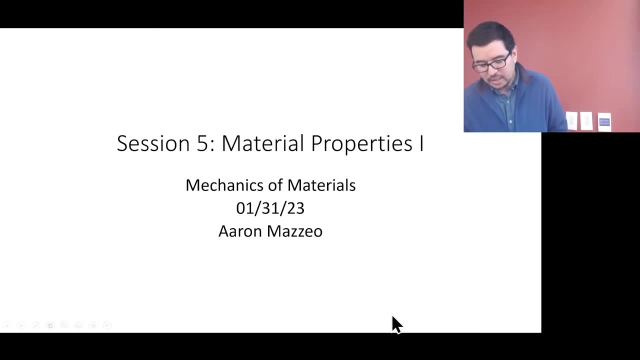 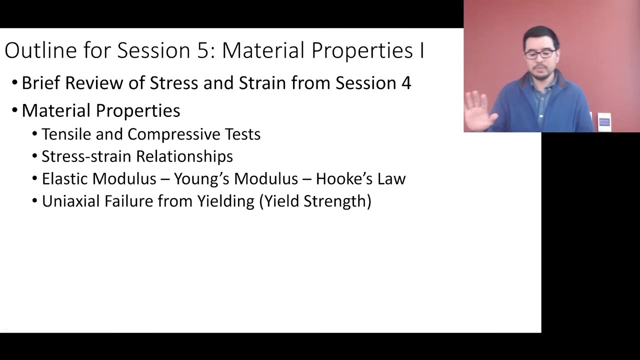 Okay, So let's go ahead. Oh, can people online hear us now? They're good, All right, Great. So today we'll do a brief review of what we covered last time in session four, And then we'll get into material properties. We're going to spend a couple of sessions discussing material. 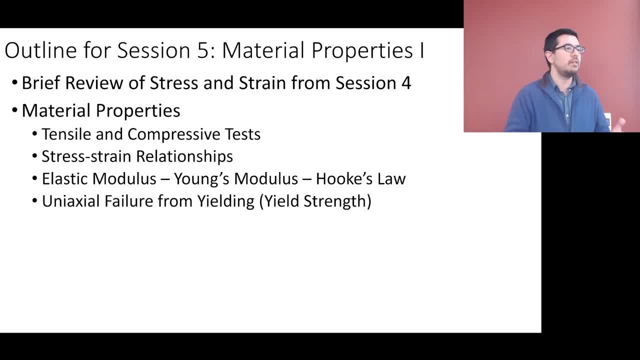 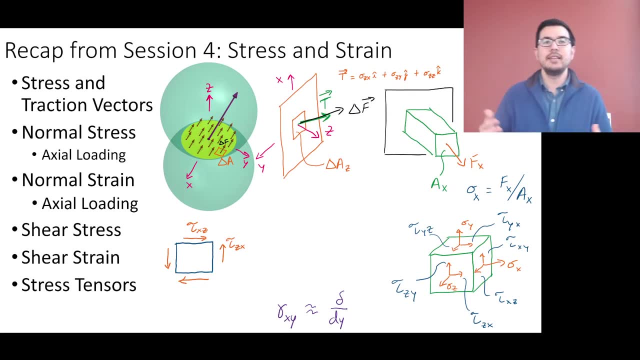 properties and how we connect them to problems that involve loads and bars, essentially, at this point in the game. The last time we met, we talked about material properties, We talked about material properties, We talked about stress and strain And we introduced some jargon. So, if you want to, 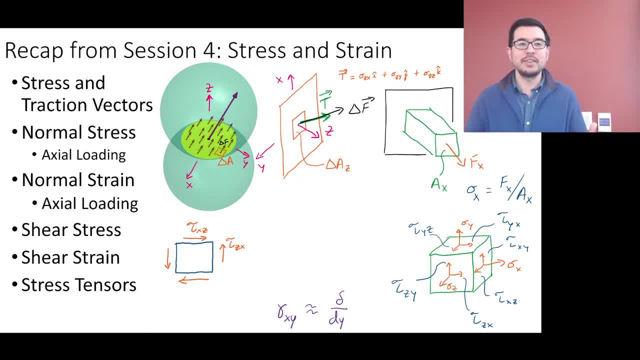 sound cool on a Friday night, you can talk about the traction vector. All right, I was like: oh, the traction vector. What is a traction vector? Well, it's a construct that we have with three components for stress, And it allows us to understand the behavior the material is experiencing. 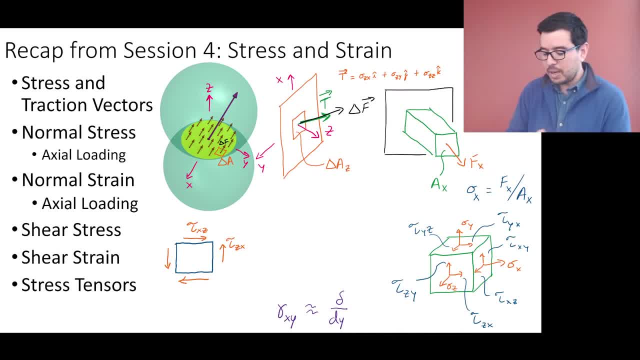 It kind of has feelings. No, it doesn't have feelings, But it is the construct that we use to take a resultant force coming out of a given plane or surface and be able to describe two sets of shear stresses, or two shear stresses and one normal stress on a given surface, And then 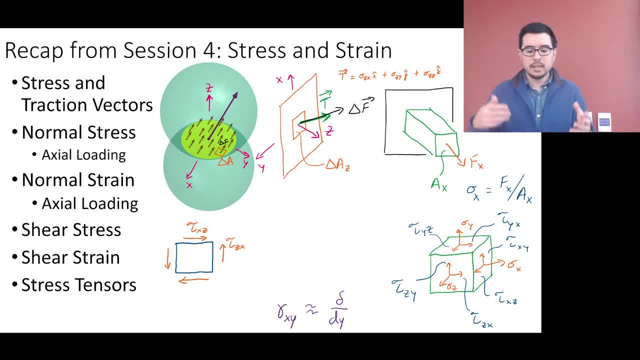 we talked about how we can have essentially six components, or if you have the tensor, nine components, But really we're going to talk about how we can have six components. or if you have the tensor, nine components, But really you have six components for our intents and purposes in this. 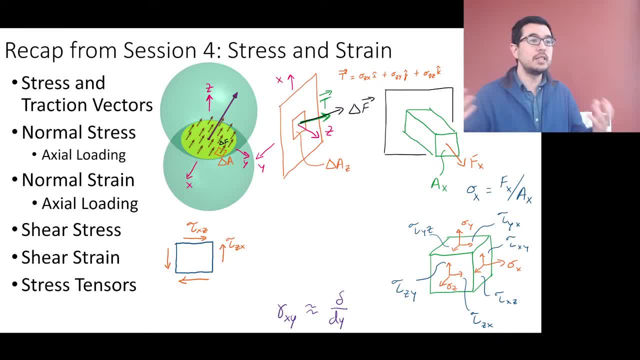 class where we have three normal stresses, sigma x, sigma y, sigma z- And we have tau xy, tau xz and tau yz, And with those stresses we're able to describe, or with those vectors that have scalar form, also positive, negative sign, we're able to describe the state of stress at a given point. 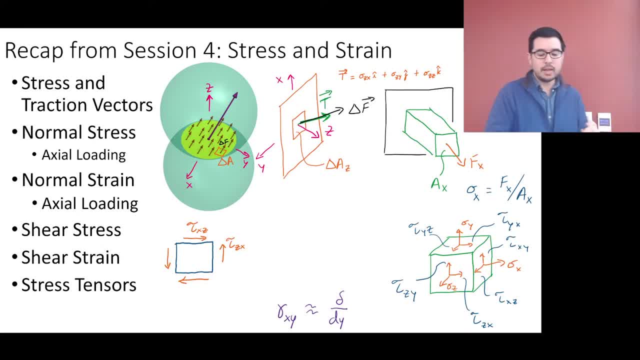 Then we talked about strain associated with axial loading. We talked about shear stress in a little bit more detail and shear strain, And we will get back to talking a lot more about shear stress and shear strain in a little bit. But first we're focusing mostly on normal stress at this point and normal strain. 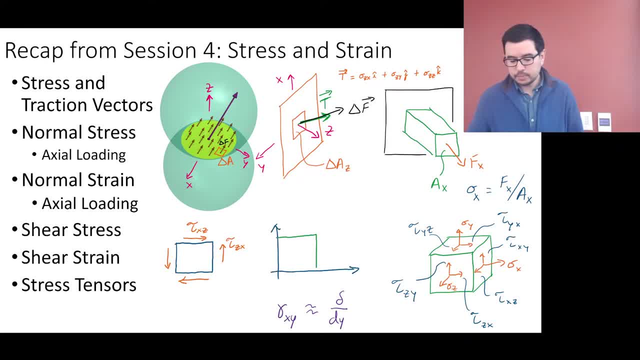 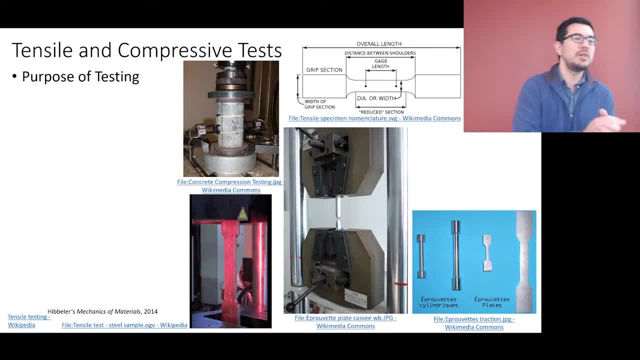 in bars. So, oh yeah, and that was the shear-shear one. All right, So has anyone done any tensile testing, material testing, Yeah, Yeah, What Do you want to talk about it? You don't have to, but what? 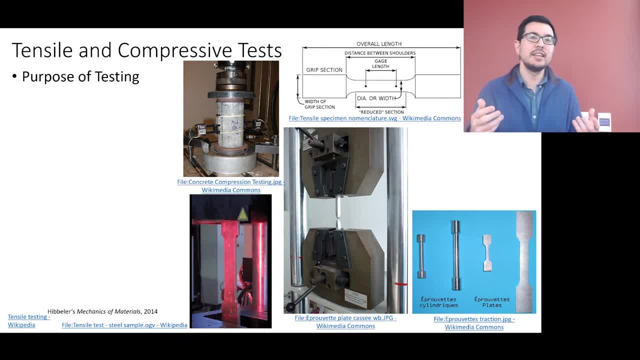 Okay, Okay, How do you impact this? Like a sharpie? No, it's not so like a metal. Yeah, Okay, All right, cool, So you're measuring in some way, shape or form, how much energy the material's able to absorb And you get an idea of whether or not it's going. 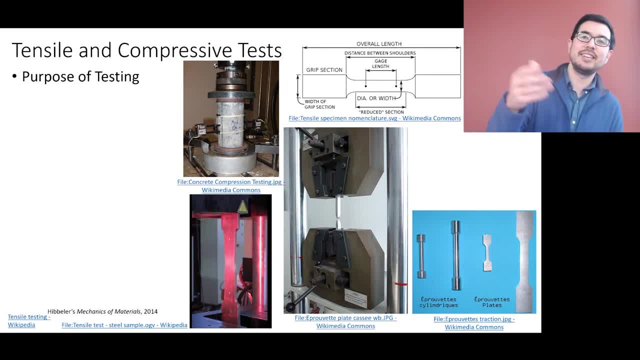 to fail when you apply that much energy. Is that what you were going to say to him? Mm-hmm? We also do another thing: edit for RFR. but we also certify our welders using the, and that's a tensile test. so we have dog bones similar to those and we cut them. 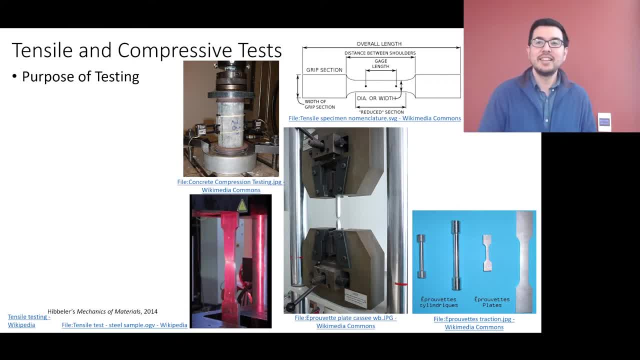 and have our welders weld onto them so that we can see if the material fails at the valve or if the material fails at the. Okay, great, So do you have a jig that you put them in to test them, or you kind of just? 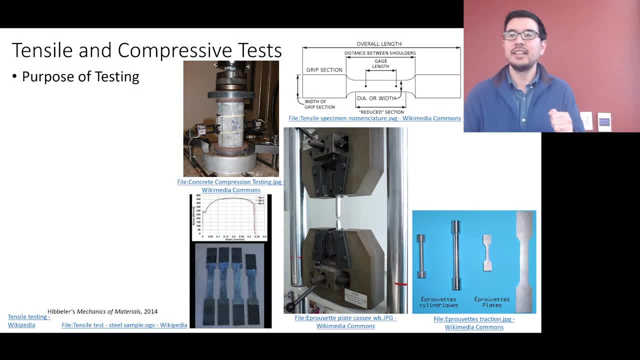 use a hammer and you're like this is not going to work. We use a. Okay, I don't know, I think Okay, yeah, Yes, yes, I'm guessing it's in Pellegrini's lab. 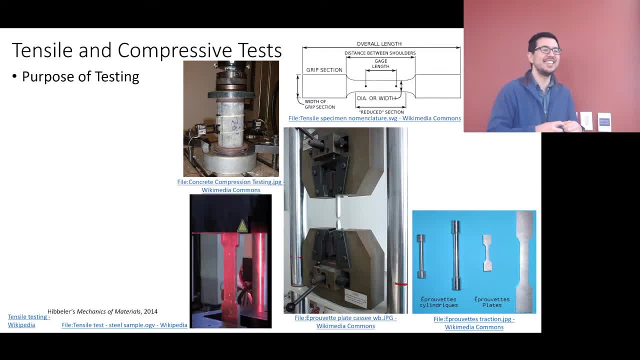 Yes, okay, good, good, good, All right, great. So you have some familiarity with what some people have, some familiarity with what material testing looks like, And if anyone's ever broken a rubber band or twisted the pin, a paper clip, you have some natural experience understanding how materials fail. 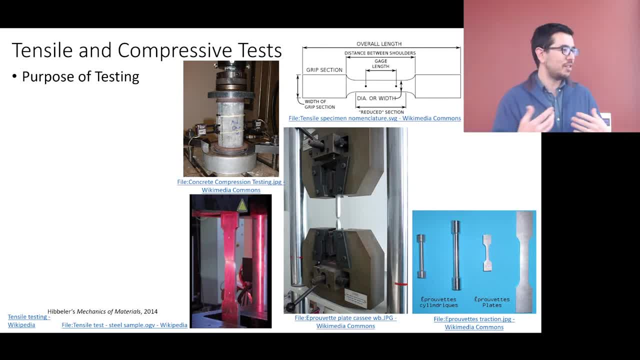 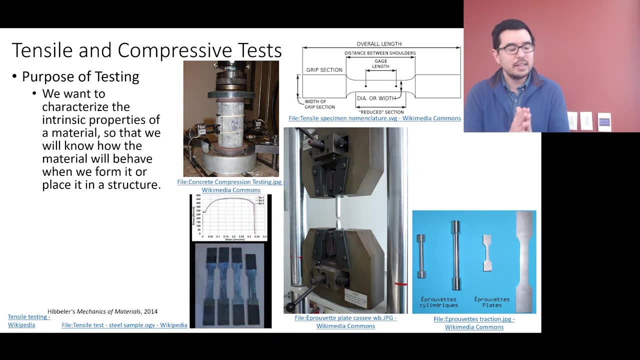 And if you apply more load or more strain, there's a higher likelihood that you're going to cause some type of plastic deformation, yielding or ultimate failure. What is the purpose of testing? Well, we want to characterize the intrinsic properties of material so that we will know how the material 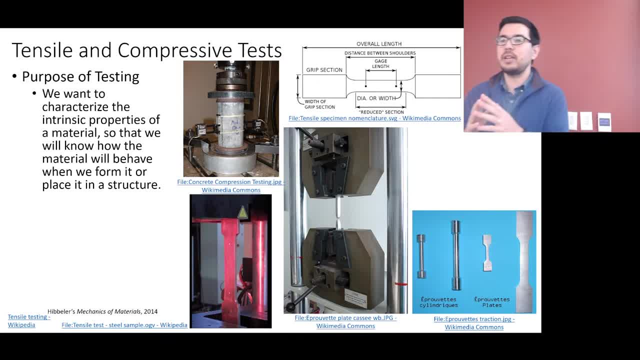 will behave when we form it or place it in a shell. So we want to understand the structure. The last time we were here, I discussed briefly how you're not going to take a bridge and put it in a material testing machine, Although there are machines that allow you to do diagnostics on structures of large size. 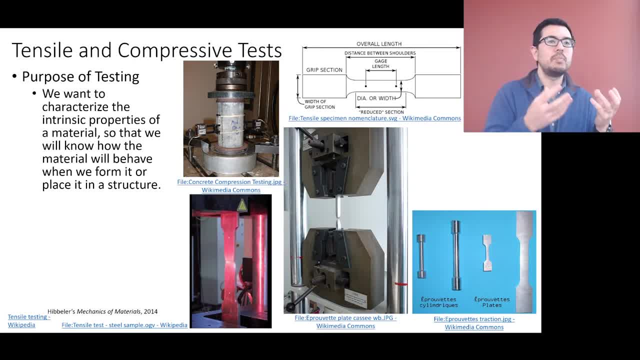 the idea is we take small pieces of material that are used in larger structures or vehicles or toys, whatever they might be, and we get an idea of how they're going to behave so that when we design, we can predict whether or not we're going to be exceeding the capacity or the strength of the materials that we're using. 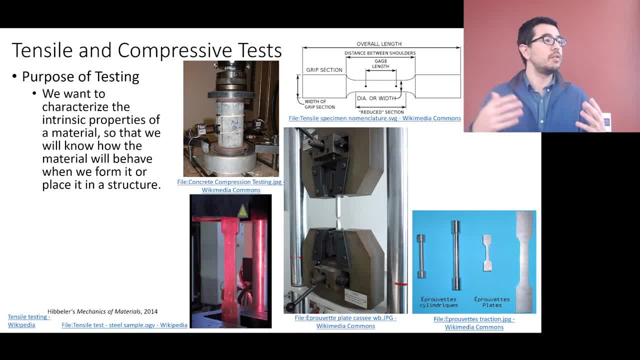 Or it could be that we're going to be able to understand how much deformation that we have and assure ourselves that we're not going to have a sagging bridge or something that's going to deflect beyond what we would like. We often use coupons or test samples. 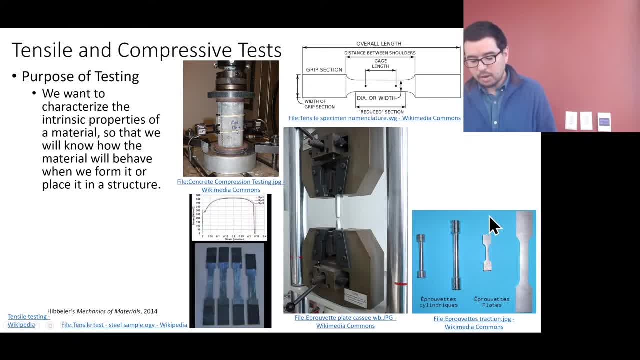 Like you see in this diagram or you see here, and they can be cylindrical, they could have threads on the ends, or they could be flat-like or squarish and have areas on which you can apply some big jaws or clamps, Or it could be a compression test where you essentially have two flat surfaces. 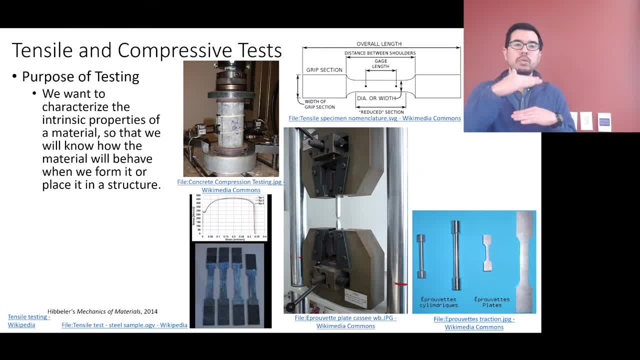 and you put it between two platens and you push those platens together to be able to generate some compressive stresses. So this is what the testing apparatus looks like. Any idea why it's wider here and here than it is in here, So it fails in the middle. 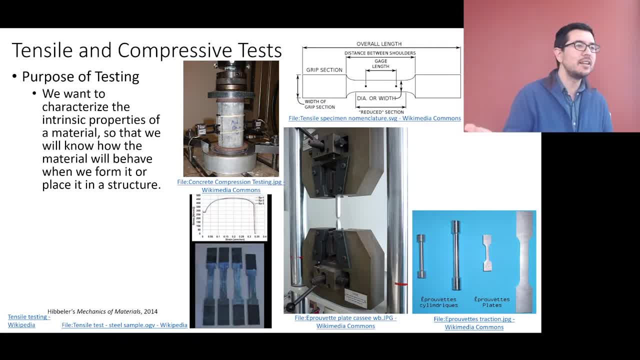 Why would it fail in the middle and not at the outside Right? it's thinner right. So we have an idea, based on our discussion of stress right, that the stress is going to be dependent on the cross-sectional area. So we want to have larger regions where you're gripping. 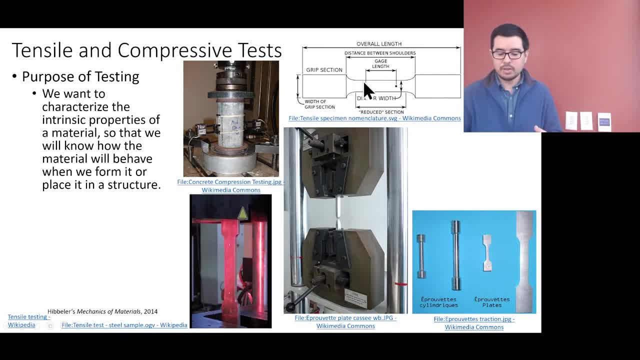 so that the failure happens in the middle. Now is it going to happen here, here, here, or here, I don't know. You don't really know. You just want it to happen in a region. But there's some randomness to this. 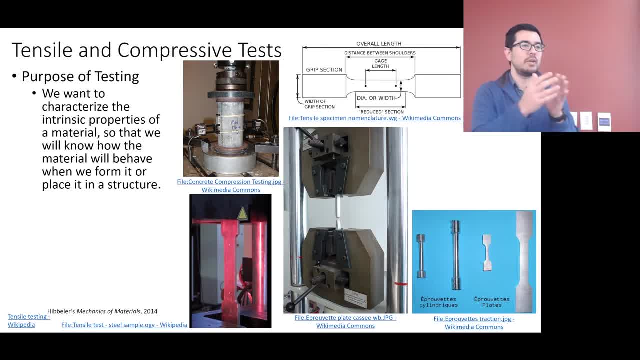 And where the defects may be or may not be. that's where you would expect or not expect there to be failure, And there are specifications- ASTM has standards on these, for example- and suggestions in terms of what the radius should be here and here and here, to avoid having a mishap. 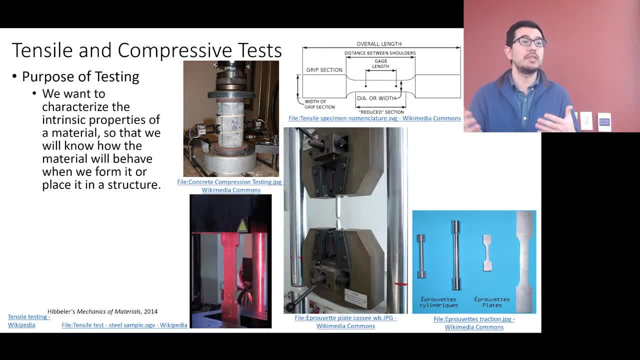 or avoid having a test fail where you don't want it to fail. Okay, As we discussed last time, we're able to calculate stress based on a normal force and an area, and we were able to relate an average normal stress to an average normal strain. 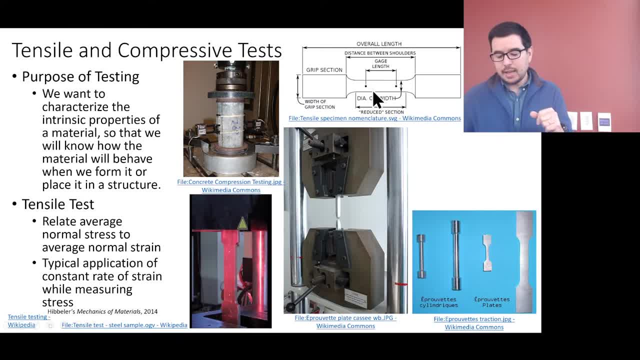 So we don't say, well, at this point it's going to be exactly the same as that point, Right, We don't. It's hard to make that prediction, But for many intents and purposes we can say, hey look. 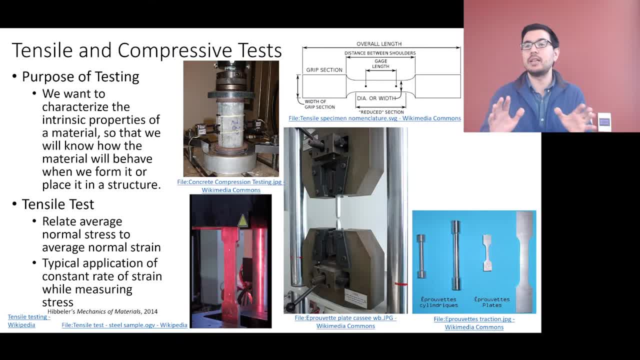 the average is going to be about right. It's going to be about the same across the cross-section And typically you or I or we would control the rate of extension and monitor force and keep that rate of extension constant. So what does that mean? 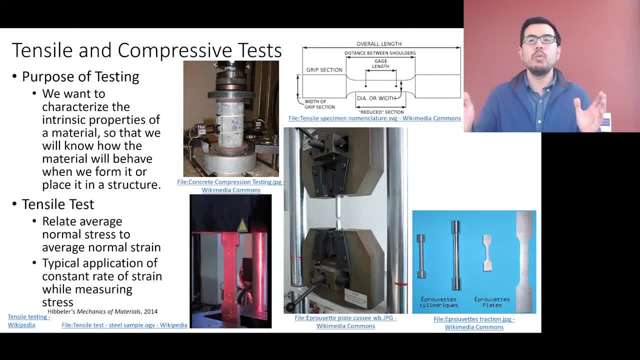 That means that we're going to be saying, hey, go one millimeter a minute, something like that, whatever it might be, And that might be a lot. Maybe we only want to go 100 microns a minute, Whatever it is, within some resolution of the machine. 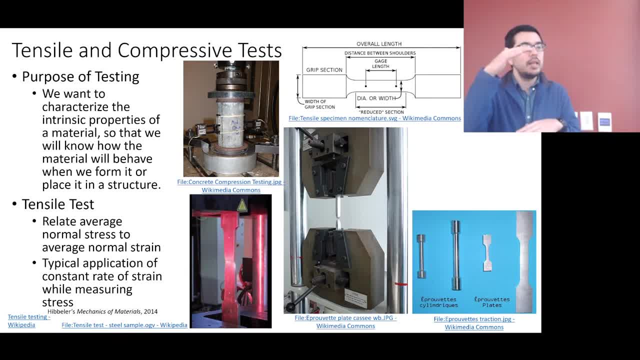 we're going to apply that displacement and we're going to measure the amount of extension, either optically or with contact extensometers, as they're called Real, original name extension extensometer, And we also need to measure the force with a load cell. 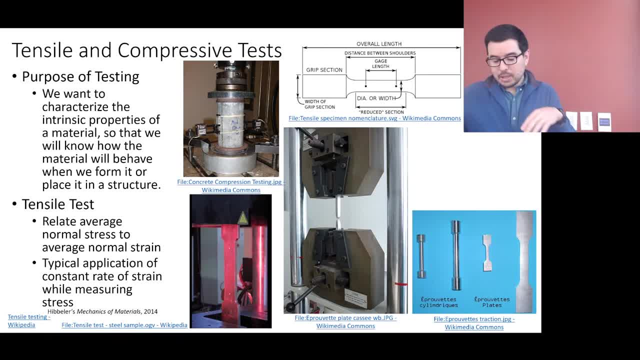 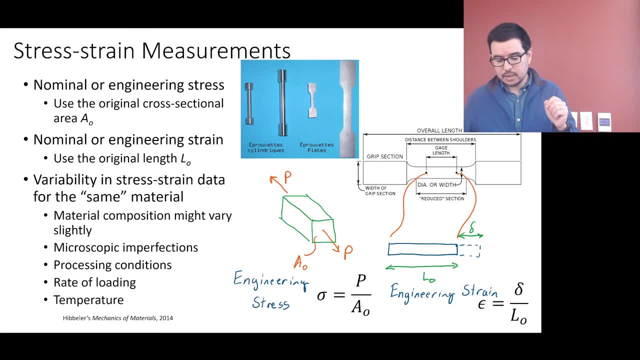 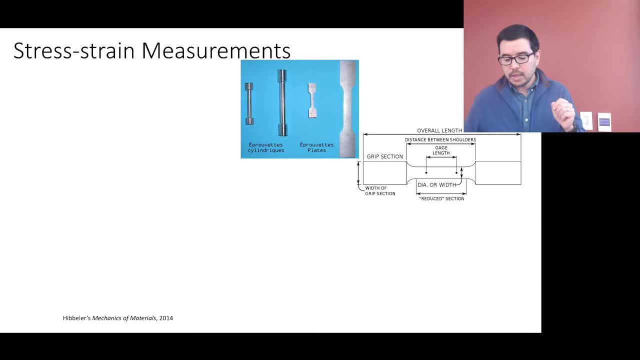 It turns out these big machines. you see that these machines have some size to them here and here Let's see, Do I have another machine? OK, maybe those are all the machines I showed. Those machines are pretty large and they need to be able to handle high loads in some cases. 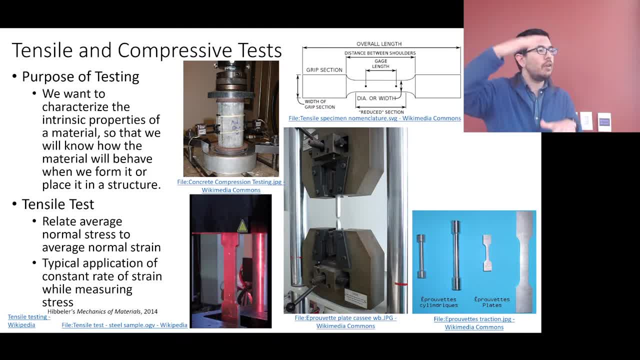 But with their size they have also the ability to flex or stretch some, And so what you want to do for more accurate measurements or measurements with high accuracy is have the extensometer either contacting the sample directly, or you have a camera that's looking at the sample directly. 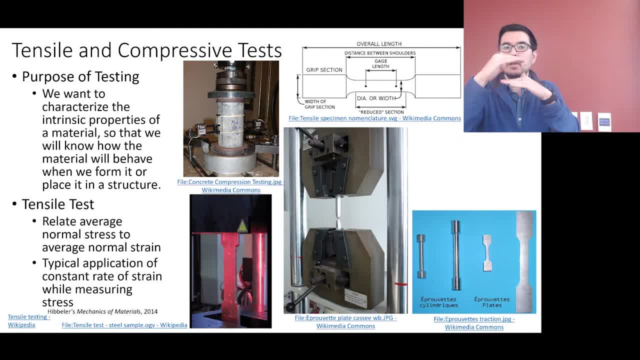 and you're measuring the distance between two points on that sample. Or you do something called digital image correlation, where they have a bunch of speckles on the sample and they have these complex computer algorithms that are able to calculate strain from the images based on the fact that all these dots are moving really small amounts. 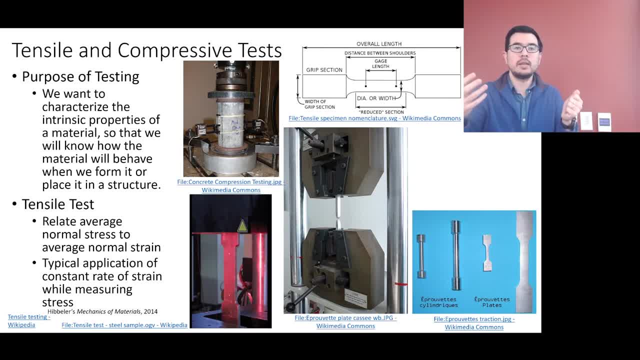 And then the load cell. that's what measures the force, And so that's going to be in series with the sample. As we know, we put springs in series with each other. the force is going to be the same. Any questions on this? 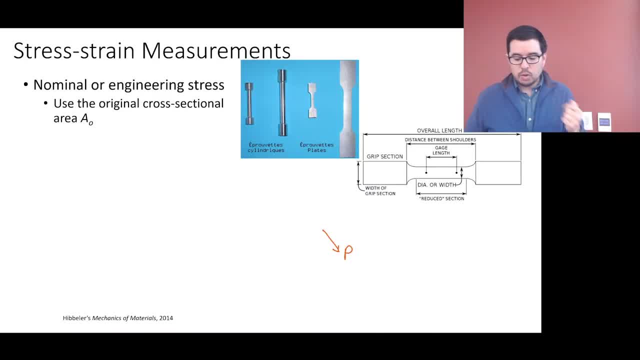 OK, So when we perform these tests, typically for metals, where we have, or alloys, where we have, small strains for a given amount of stress, we use what's called the engineering stress, And the engineering stress is based off the original cross-section. 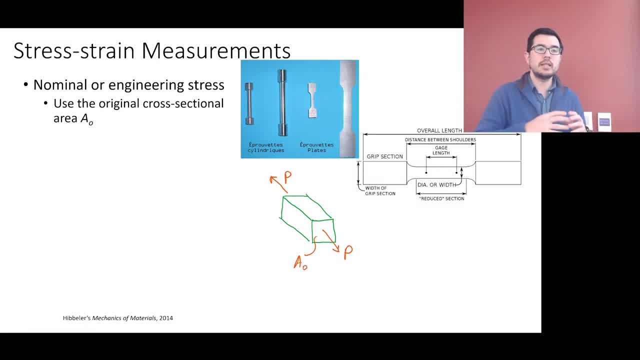 We'll call that A naught. So you have some force and it's scaling up, but we're going to assume that the cross-sectional area is more or less staying constant As we'll discuss on Friday. not true, but again, it's typically pretty small. 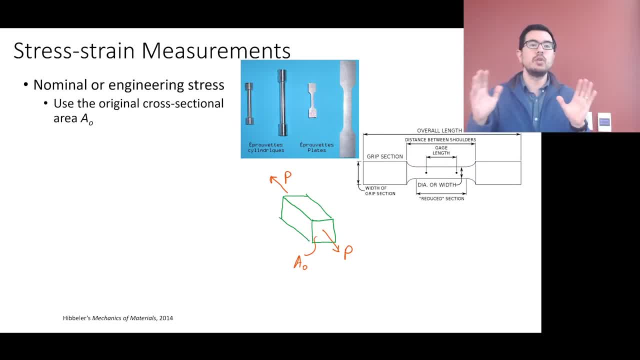 for the types of displacements and strains we're discussing. so it's not bad If you're using a rubber band or something that's rubbery. then you're probably going to want to use other methods of measuring the cross-sectional area to get a true stress. 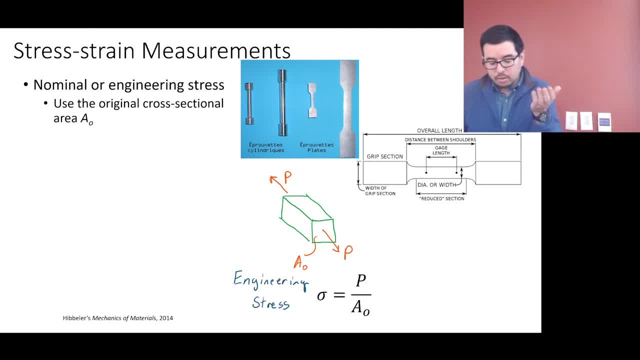 So the engineering strain is essentially- or sorry, engineering stress is just this force divided by the initial cross-sectional area. The nominal or engineering strain is going to be based on the original length. So we're going to measure that length and then say what is the little delta. 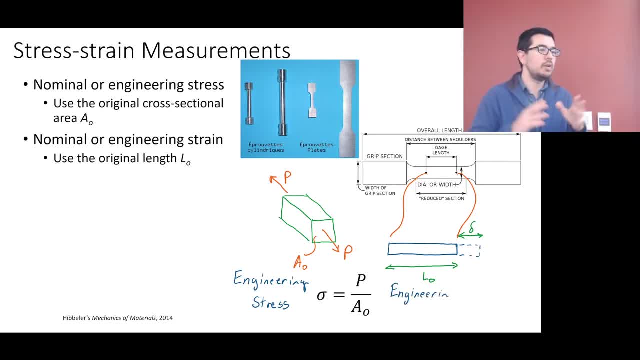 and that little delta divided by L naught is going to give us the strain Again. there are other ways of calculating strain And this is typically good enough for this class for what we're going to be discussing. You try hard to set up these experiments. 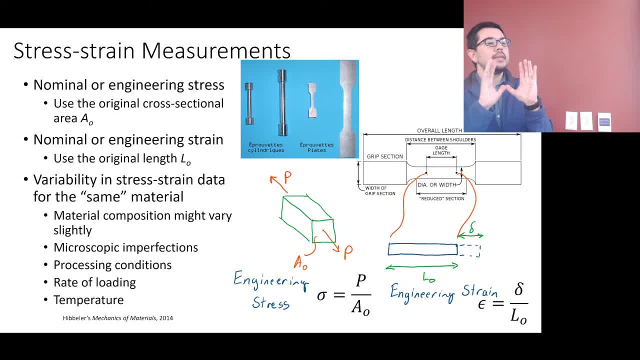 and be very careful with the instrumentation. have a great load cell, have a great extensometer. What does that mean? What does great mean? Well, it means that the level of noise you have is low compared to the minimum amount that you're going to measure, right? 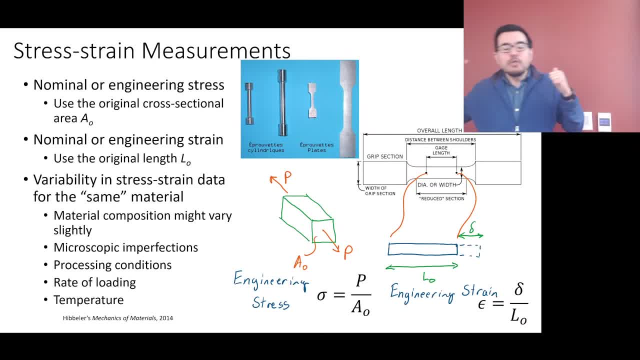 So someone says, hey, I've got a five kilonewton load cell, Do you want to use it? And you're like, my sample is really small. It's a small cross-sectional area. It has a low elastic modulus. 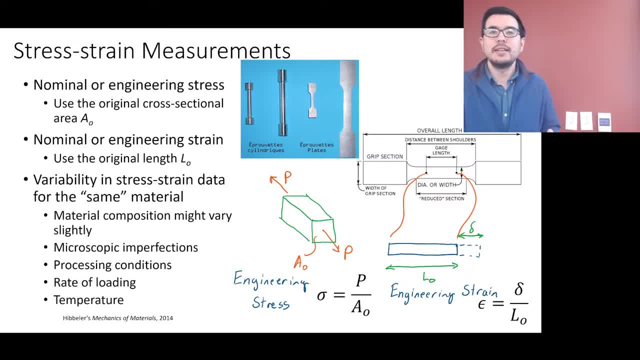 I only need 100 newtons of force max. Well, let's just imagine that both the 100 newton load cell and the five kilonewton cell have a range between 0 and 10 volts for their output. okay, 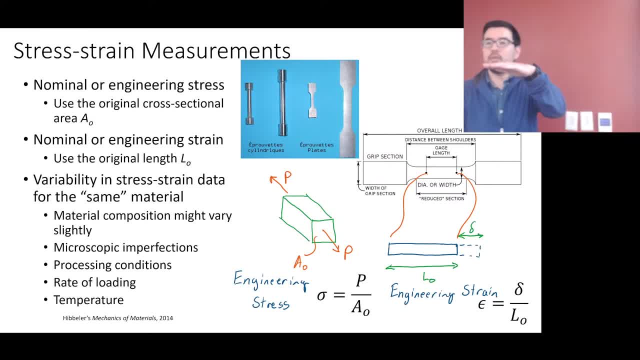 So that means that the 100 newton load cell- right, you're going to have 10 newtons per volt, okay- Whereas the five kilonewton load cell- right, that's 5,000 newtons over 10 volts. 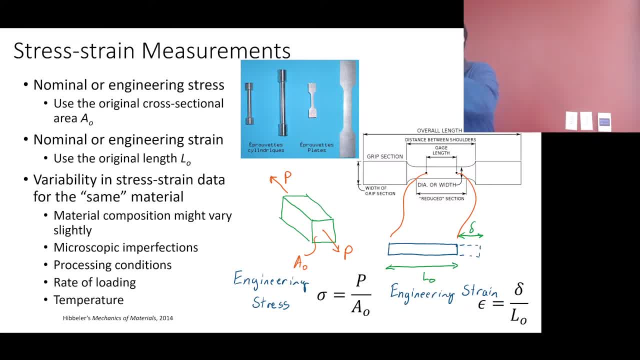 That's 500 newtons per volt. okay, And let's just say that there's noise in that voltage signal. If you're trying to measure three newtons, the five kilonewton load cell may just spit out noise. that's going plus or minus. 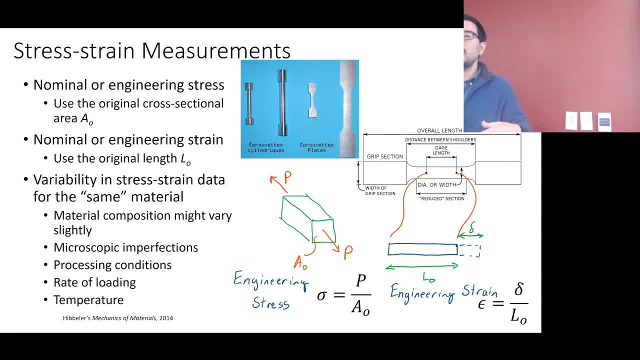 five, 10 newtons all the time, okay, Whereas the 100 newton load cell will be able to give you a more stable readout and probably get you down to the three newtons. Does that make sense? So bigger is not always better, right? 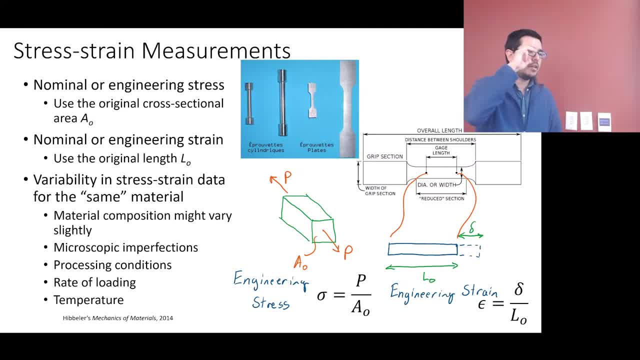 And accuracy and resolution and repeatability are all factors that go into being an experimentalist trying to do careful characterization of a material or a process. Temperature can also affect your measurements. We won't talk about temperature much in this class, at least from the perspective of 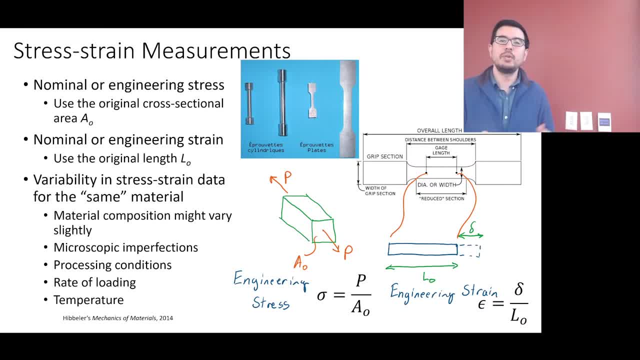 how does the elastic modulus depend on it? We can talk about it a little bit with heat treatment and things of that nature. but when you take mechanics or material props, properties of materials, they'll talk more about how the microstructure evolves and changes based on the quenching. 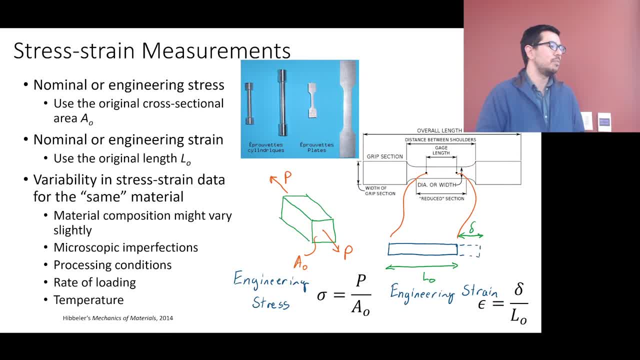 or the annealing processes that might be in place. So we're going to kind of just say: hey, here's your elastic modulus, have fun. And yes, a little microdense or voids can end up leading to imperfections and issues. 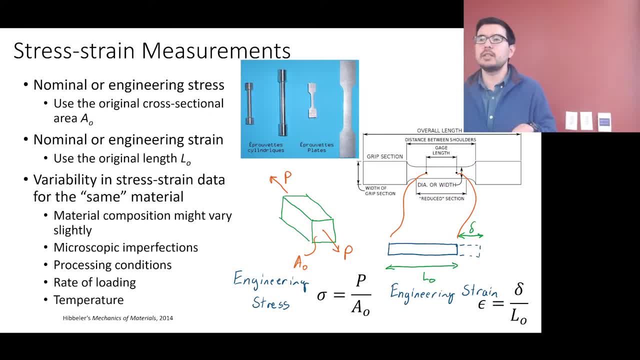 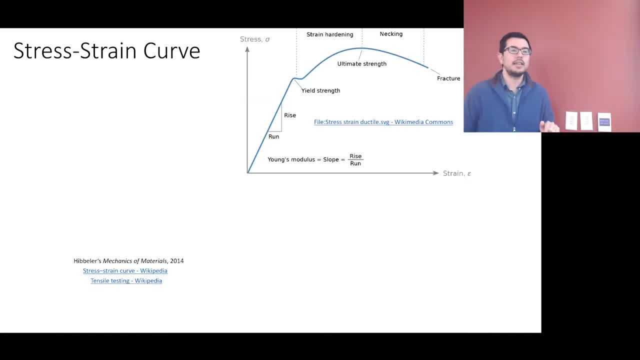 with your tensile testing as well. Okay, any questions on this? Good Fun, All right. So what do you get out of the machine? Well, we're going to go into more detail in terms of how you make a graph and how you calculate some of these values. 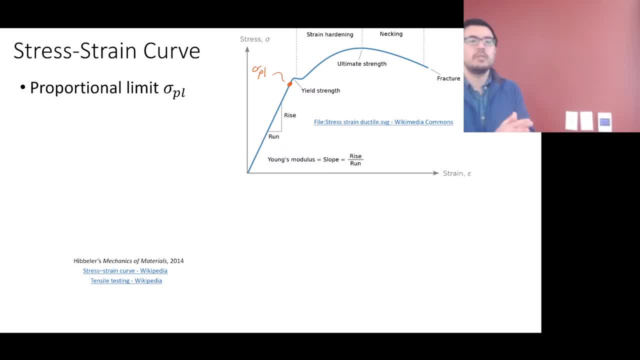 But this is what you're looking for when you're interested in using a material in an engineering application, You're looking for a plot that has stress versus strain. So the units of stress are force per area and the units of strain are dimensionless. 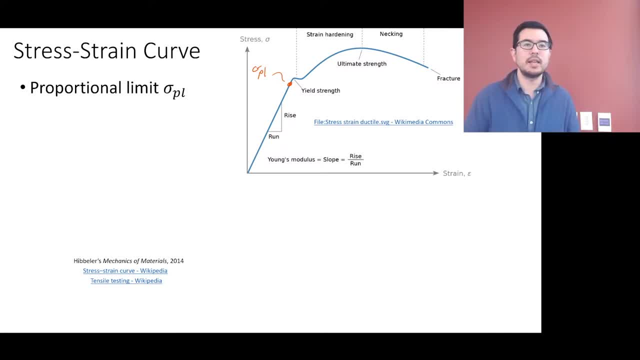 But maybe they'll say, oh, this is going to be a microstrain, right? We discussed this last time. Maybe this is going to be in percent, But it's dimensionless. Now, one point on this stress-strain curve could be the proportional limit. 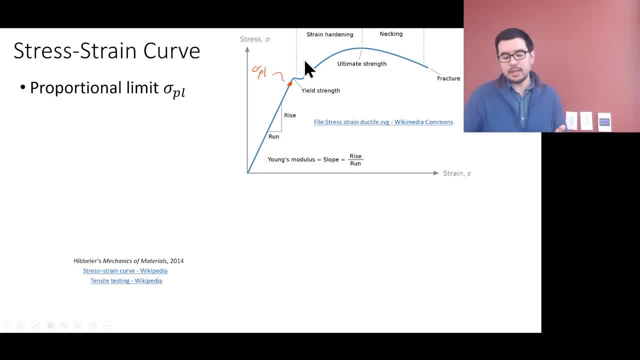 And there are going to be a few values here at the beginning that are almost right on top of each other and so often we don't distinguish them. But the proportional limit is saying: this is a point through which I can draw a line and I have a constant of proportionality. 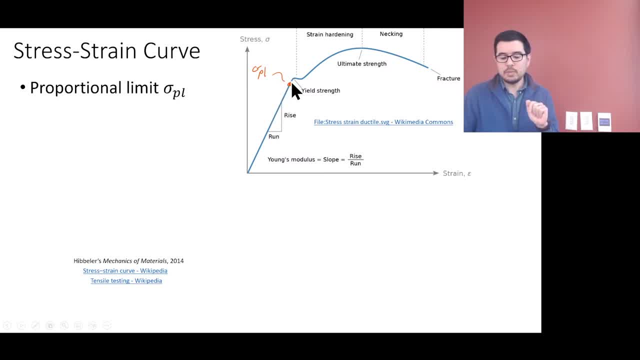 Okay, So after I get to this point, okay, it could be here. I mean this is not super precise, right, But it could be here, It could be a little bit here, Whatever, It could be down here Okay. 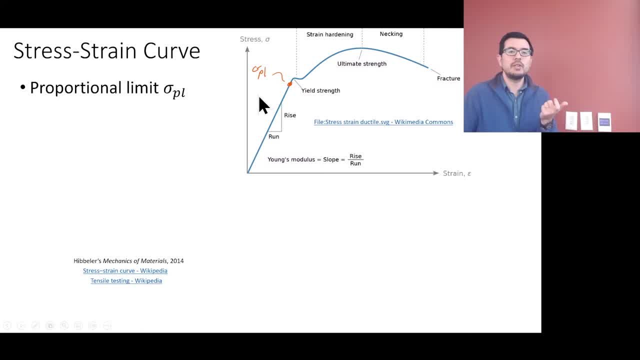 I start to go nonlinear. Right, People like that term nonlinear- but you can see this is a line. This is something that's not a line. Okay, At least you know it has some other behavior. The elastic limit: Okay. 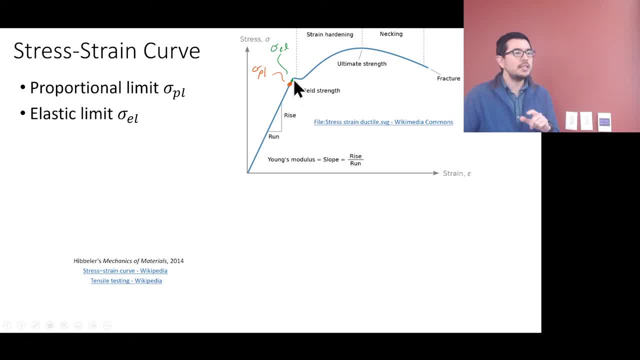 Elastic limit could be a little bit higher, and the elastic limit is the stress to which you can go, and when you unload, you spring back all the way to zero. Okay, So this is a key point in design: We want to keep the stresses low enough. 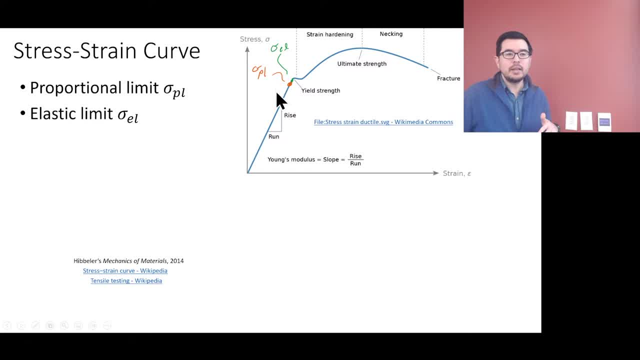 so that when they are applied and when they are released there is no resulting deformation. Does that always happen? No, Obviously, But that's kind of the typical goal for a design engineer. The yield, stress or strain, Okay, So this point right here. 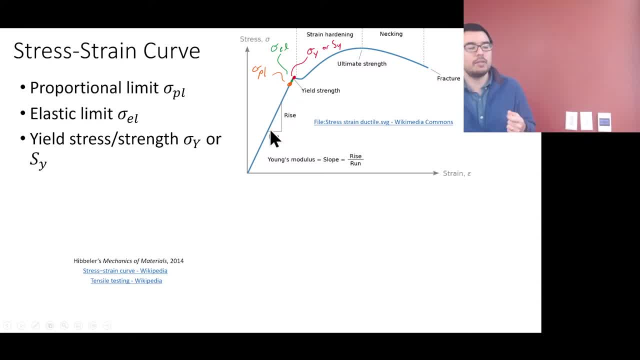 a little further up, given by sigma y or sy, is very similar to the elastic limit, And they could almost be on top of each other. All right, But the yield strength is. once you get to that yield strength, you will no longer go back to zero. 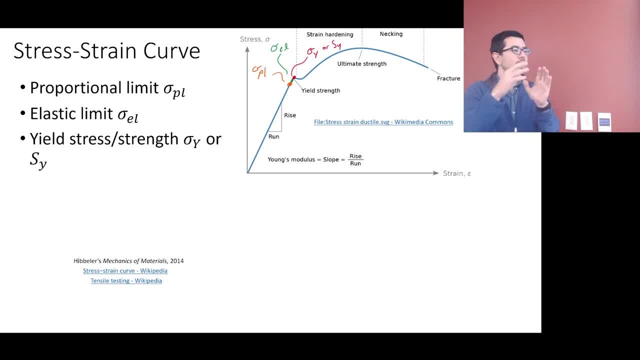 Okay, So again, the elastic limit or the proportional limit. the elastic limit and the yield strength are often just assumed to be at the same location for most intents and purposes. We'll discuss a little bit about how you might calculate a yield strength. 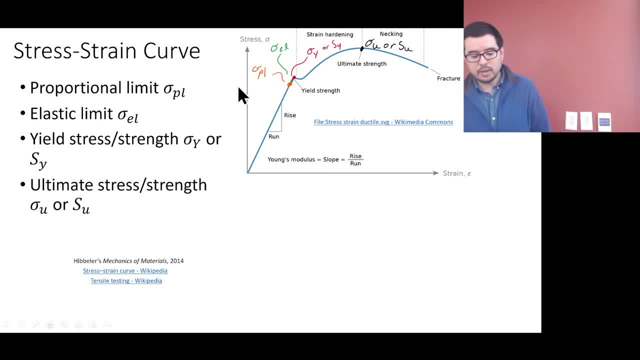 though later. The ultimate strength or ultimate stress- okay, out here is, as you guessed, the maximum stress that the material will handle. You don't want to be operating out here usually, Okay, And what you see is that the slope. 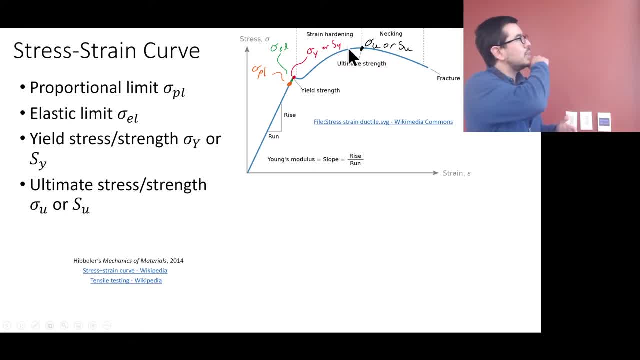 falls off and kind of becomes flat. You know what that means. when it becomes flat, That means that if you keep applying the same amount of force, which is the same amount of stress, the material keeps straining. Okay, Now there are situations. 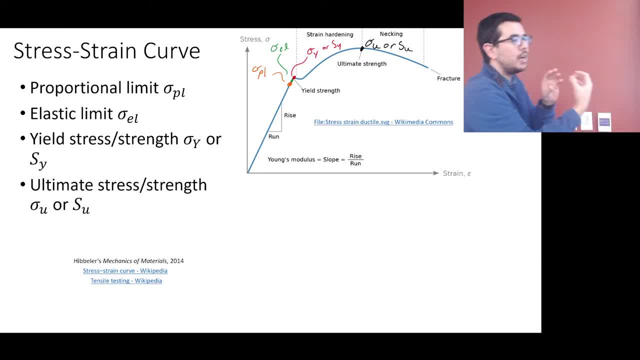 where you have polymers that creep and different things of that nature, yes, but this, when you're dealing with the metallic alloys, this is a big-time no-no. Okay, Big-time no-no. You want to be down here, Unless you're trying to break it. 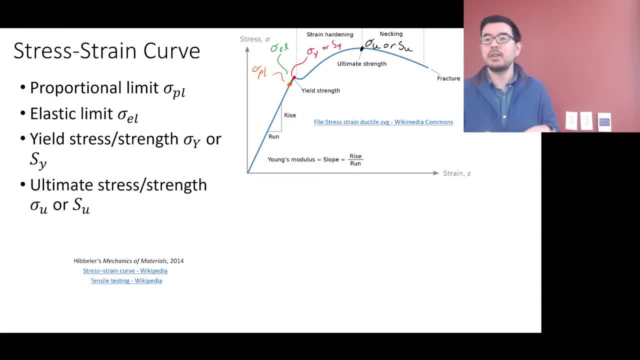 Okay, Maybe you have a system that you're designing where you want the user to be able to pop out their gum from a package, Right? So you've got this really thin piece of metal there. So you actually designed it so that it does fail. 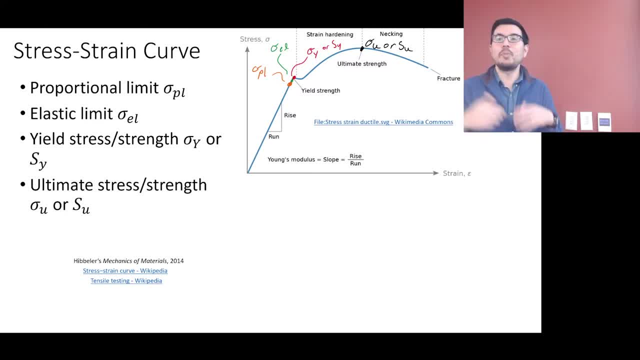 Okay, And that it's not too hard to open Or a bag? Right, Some of you are probably packaging engineers, right? Do we have any packaging engineers, Okay? Well, if you were a packaging engineer, you're breaking stuff. 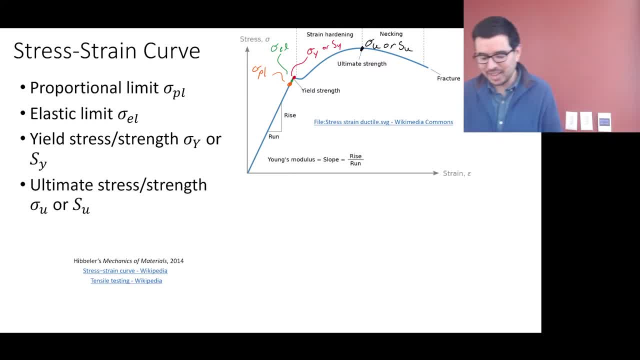 Okay. And then the last one is the fracture stress: Okay, Sigma F. And this is where, yes, we've gone beyond necking, which we'll show a little bit in more detail, Probably more. actually, I'll talk more about that. 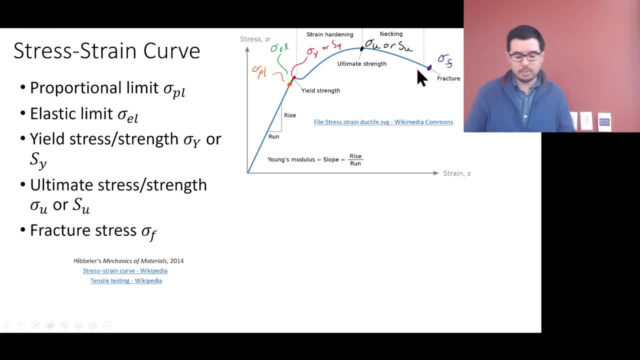 I guess on Friday, if I have time And that will you know, we'll talk about that a little bit in more detail, Probably more. actually, I'll talk more about that, but that will. that's when you break. 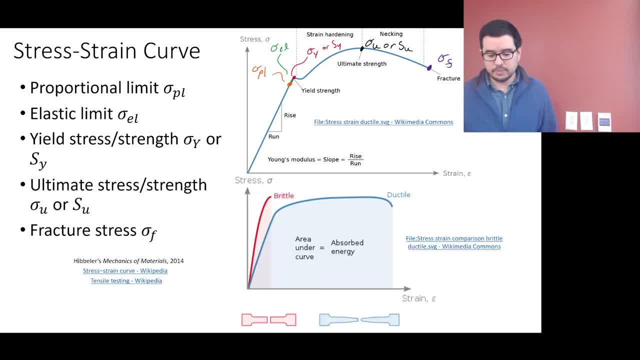 Okay, That's when you rupture, That's it Okay. So, like necking, you can kind of see it here. All right, These samples. they had a cross-sectional area then they kind of tapered out, they thin. 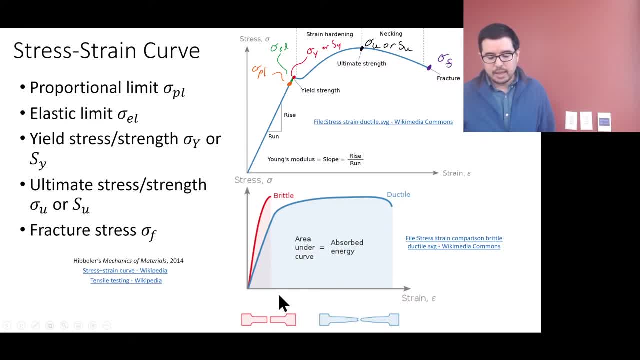 and then they broke. Okay, And there is a difference between a ductile material and a brittle material, And if you look at some of the videos I posted, I wish some of these videos existed when I was taking this class, because I think 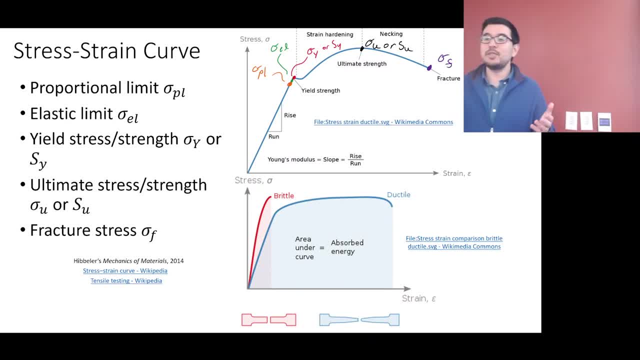 they do look a little bit different. So if you look at some of the videos I posted, they do a better job explaining graphically the principles than I can with my hands or my voice, Okay, Or my drawings even. But 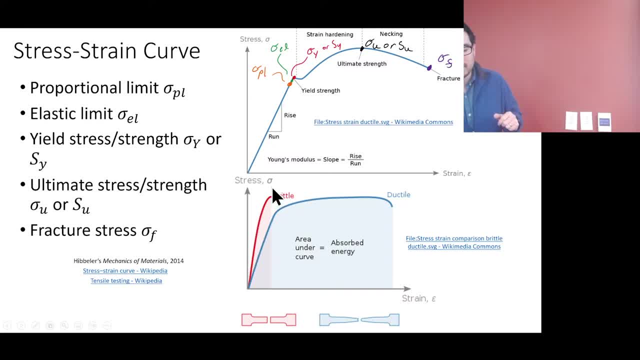 a brittle material is a material like you see here. it just- and I guess that's something to be noted- right When we when the curve ends, sometimes people put an X there. All right, That's it The material. 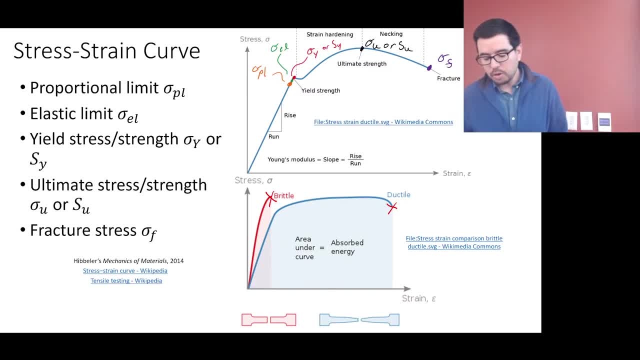 has ruptured, It's broken. So brittle materials, they have typically kind of a more sudden catastrophic failure. They snap. All right, Imagine glass, a ceramic, something of that nature. All right You, you throw a rock at it. 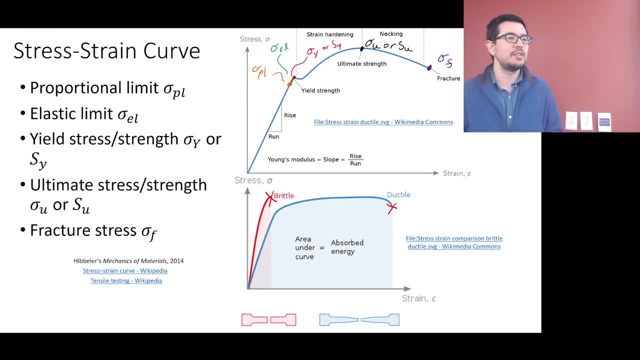 and it just shatters Something metal, like the hood of your car. right, You throw a rock at it and it puts a big old dent in it. Okay, That is an example of ductility, All right, So so. 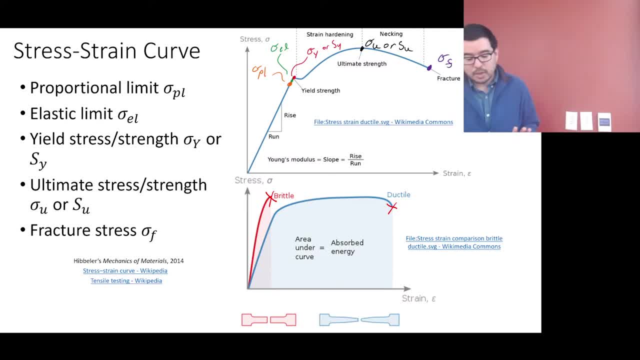 and and so, whoops, What you, what you have here also- and we'll talk about this more next time- is an opportunity to measure the energy under these curves And, like you all were talking about your impact testing. 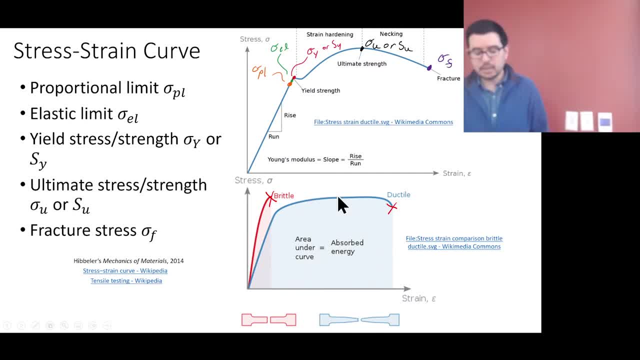 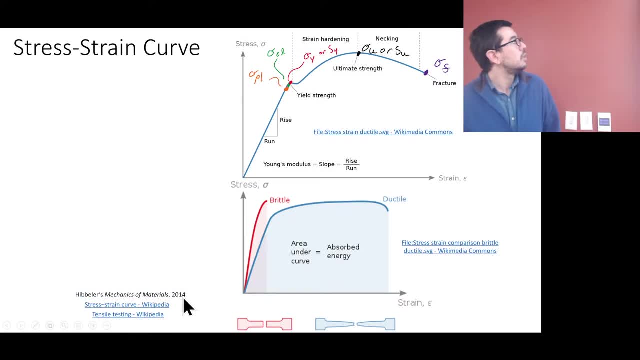 I think, With the impact testing, you're going to be looking at this property here, How much energy it's able to absorb. Okay, So some points that we already might have discussed too. It's often very difficult to distinguish between the. 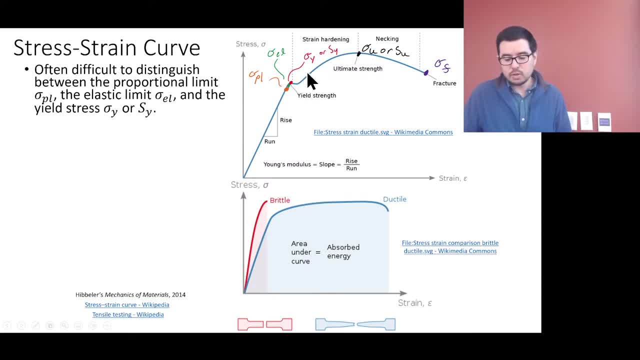 proportional limit, that's this one, the elastic limit and the yield stress or yield strength. Okay, There are two overall behaviors. One is what we call elastic behavior. So elastic means it springs back. Okay, So it's in this. 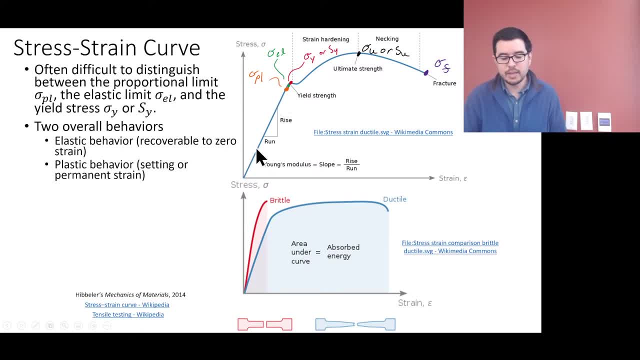 linear regime. I have to watch what I'm doing. It's in this linear regime right here And there's plastic behavior, Okay, And you have what we'll call setting or permanent strain, And I need to talk about that. 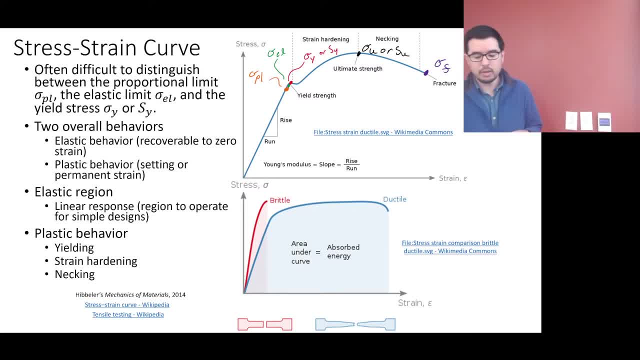 later. So elastic behavior has what we call yielding Okay Or strain hardening. So the material is actually getting harder, And I'll explain that a little bit too. when we start drawing some curves at the end of today, 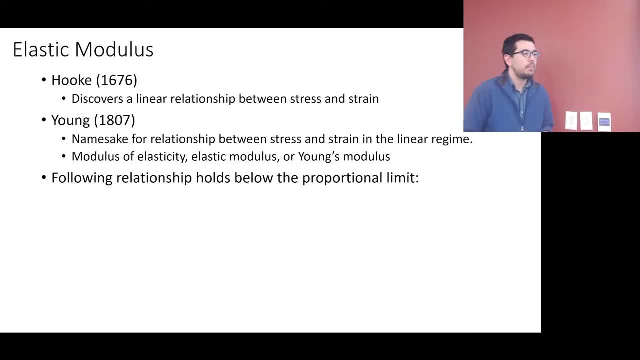 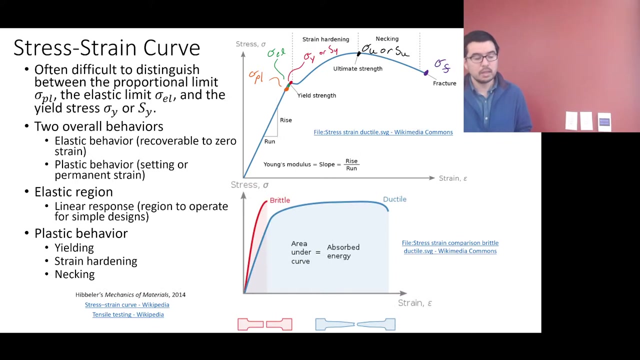 And we'll talk about that later. Now for the next little bit, let's just focus on the elastic region. Okay, So that's that linear response region, And we're going to talk about that in a little bit. 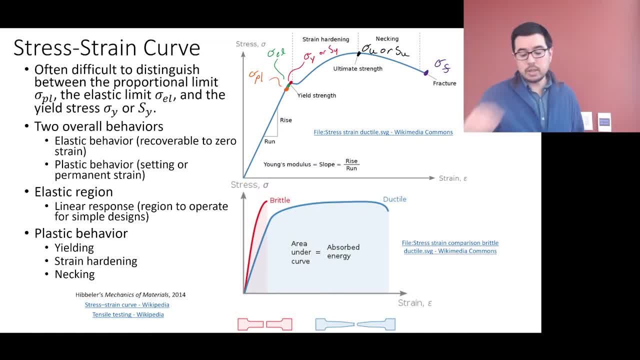 Okay, this Okay. So not all materials do this, But low carbon steel is one that shows a definitive yield point. And if you get to a point, if you think about these atoms or molecules having their interatomic or intermolecular 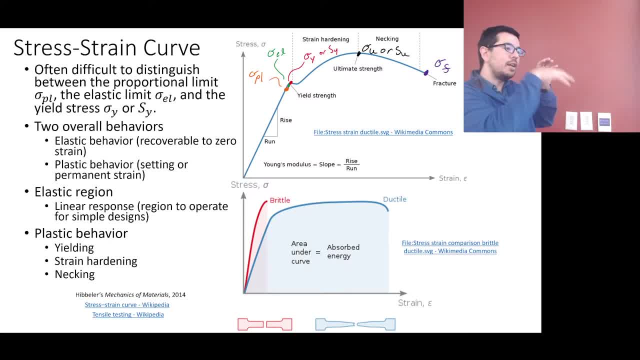 forces where you kind of stretch things out and either dislocations or other things can kind of creep in or things start to break and they slide. So stress or, I'm sorry, a strain, okay, it actually goes down. But 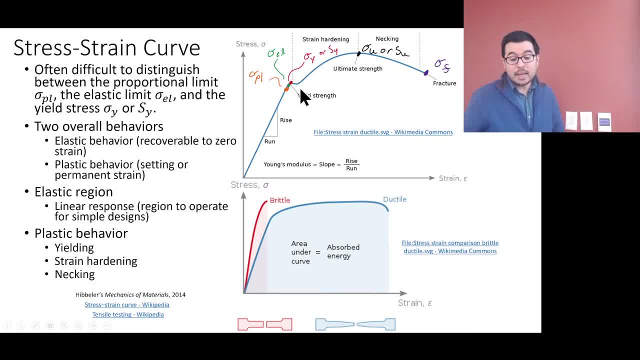 this is actually a pretty complicated phenomenon that we won't go into right now. Yeah, then it hardens. Yes, that is true. Okay, and so you can introduce what are called dislocations that actually make the material stronger, Okay. 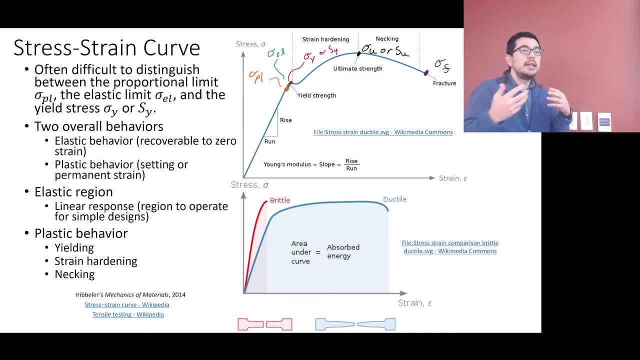 and so this is one of the wonderful things about steel and some of these alloys is that you're able to increase the strength of the material by purposely plastically deforming it. Okay, so like, if you want to do this, you can. 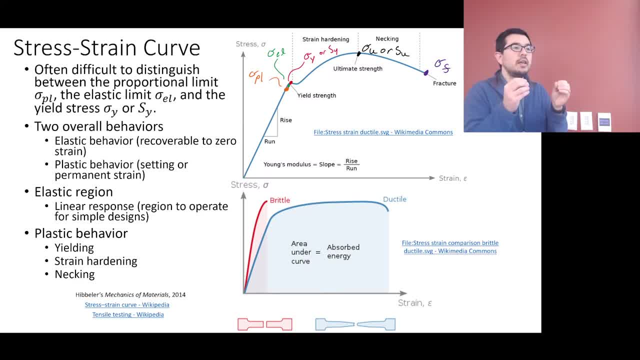 do this with heat treating, for example, to make the outer edges of the sword very hard, Okay. and like a blacksmith might be doing some stuff where they're pounding it and heating it, Okay. where the outer edges become very hard, okay. 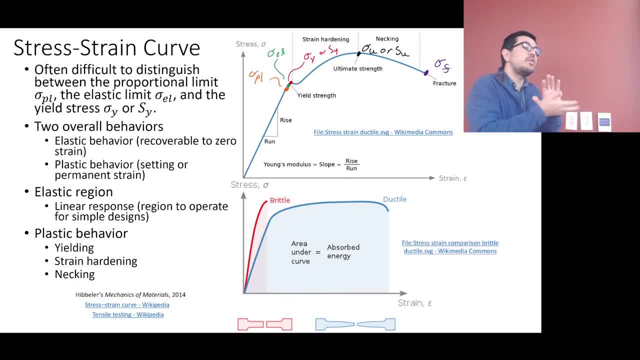 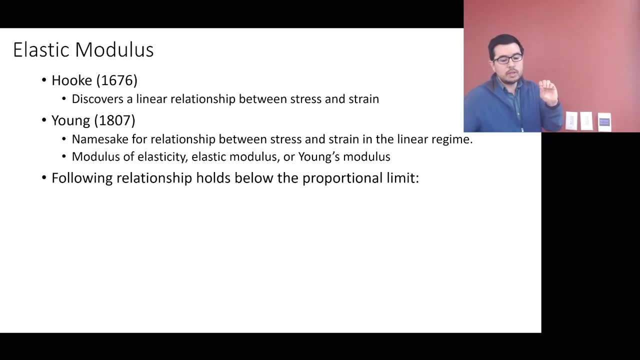 so metals are really cool. same. you started with the same material, but how you processed it is giving you different attributes at different locations. Okay so, elastic, we're in the elastic regime. okay, this linear regime, and we've talked about. 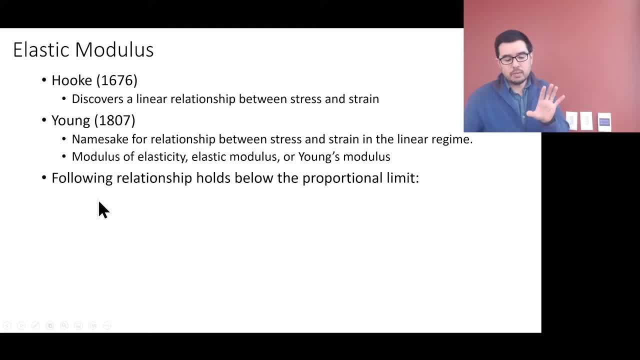 Hooke's law. there's another form of Hooke's law, which this definitely goes on your formula sheet. there's a reason why it's so huge. okay, sigma equals E, epsilon. now, what is E? E is the elastic. 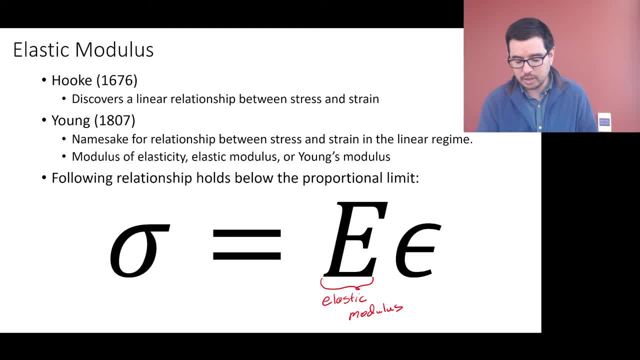 modulus. okay, this is the elastic modulus or the elastic modulus okay. so what is the elastic modulus? What is sigma? We already know what sigma is. sigma is the stress, and these are normal stresses, and epsilon is the. 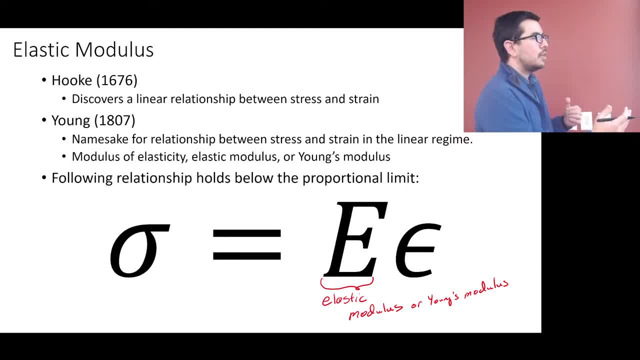 strain. so epsilon strain has dimensionless units and stress has units of force per area, which means that the elastic modulus is going to have units of force per area. Please keep that in mind. So how do we determine an elastic? 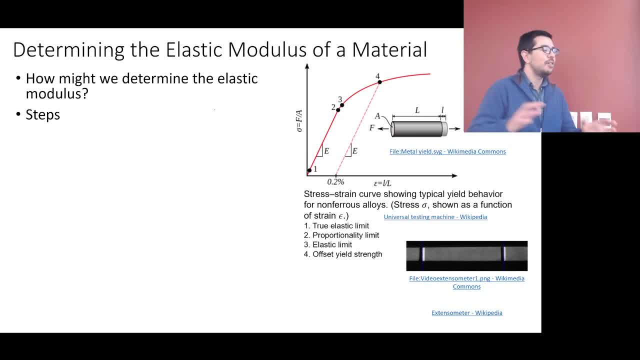 modulus. I was in a meeting recently and one of the faculty students went to an interview recently and they're asking in the interview: how do you calculate the elastic modulus? And she didn't tell me whether or not the student got it right. 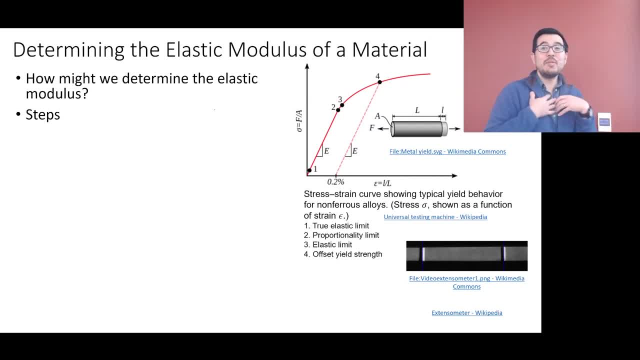 but apparently the other interviewees were kind of stressed about this question, okay, And I remember the guy that walked out right before he went into the interview said I couldn't remember the difference between stress and strain, okay, So these concepts- 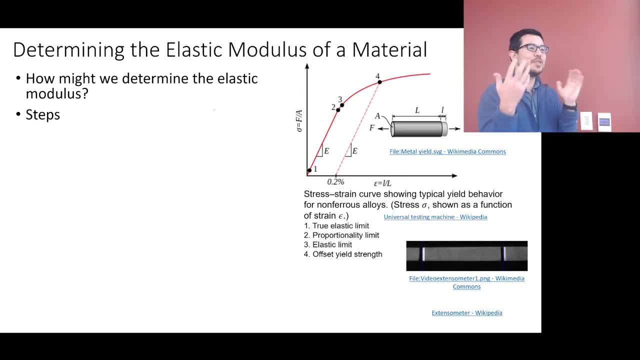 are valuable, not just because they're interesting, but you might actually need to know them for a job or some other opportunity in engineering. After that conversation I thought, okay, I gotta since, and I'm like, oh boy. 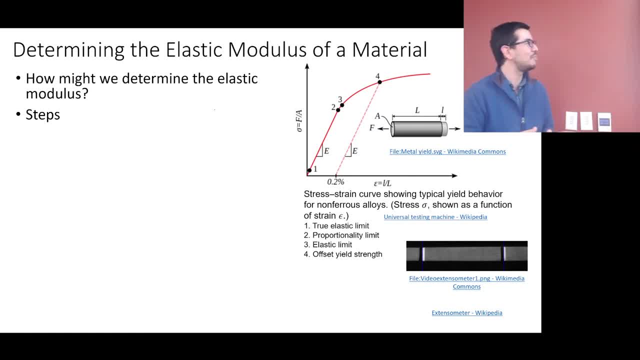 right? who's been teaching mechanics and materials right? So let's make sure that we know how to calculate an elastic modulus, And here are some steps that we can do. First, go ahead and fabricate an article, a test article. 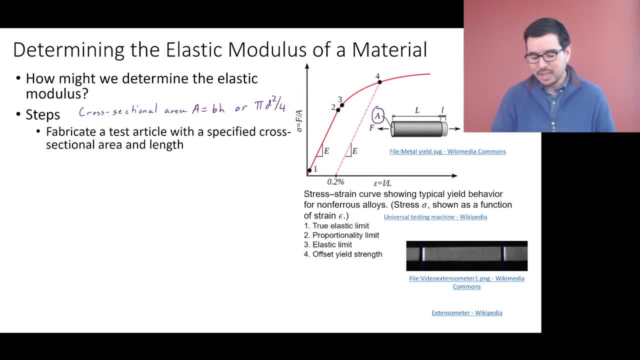 right, You wanna sound fancy. I'm gonna use a test article. I'm gonna make some samples And you want them to have the same cross-sectional area and you want them to have the same length. I didn't put that in the 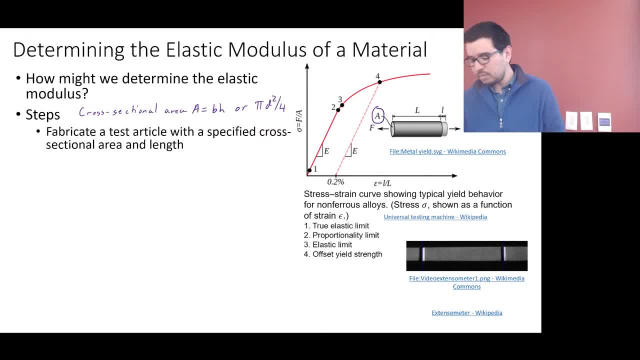 article. but you want to be able to calculate a standard deviation, you want to be able to calculate a mean. you get some idea of how uniform the material might be. Now next, after I figure out how it's going to work, 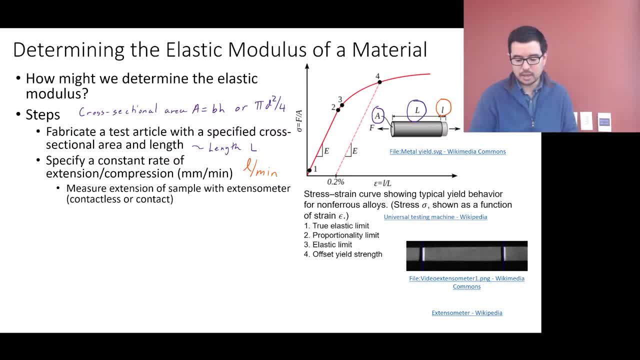 I'm gonna use a test article or if it's an extension test and I put L per minute, That's actually probably not the greatest. Maybe it should be length per time, just so that L is a length. time is a time. 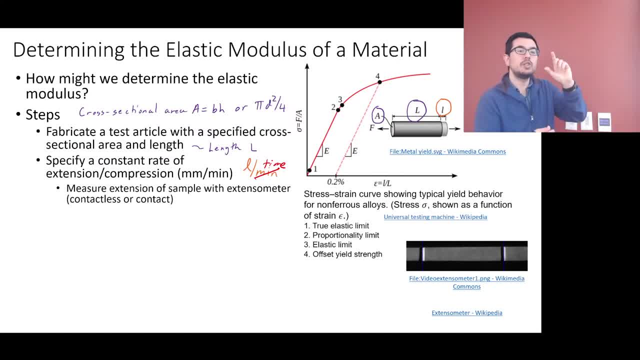 right, But you need some way either to measure the extension with a video or images or with an extensometer Or, to be honest, if you don't really care that much, you're not too concerned about the precision and the. 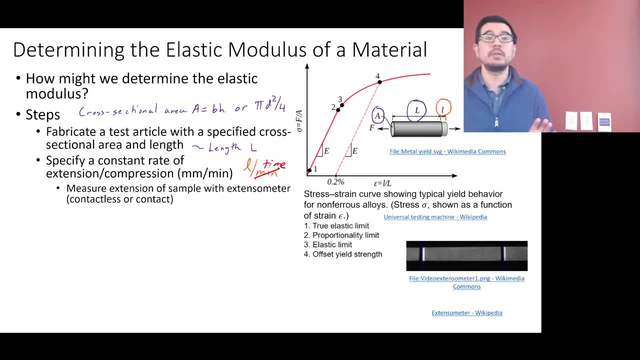 machine's not too big. you'd just be like: I'm going to test this machine and the machine is going to be quite large and the machine is quite stiff relative to the polymer that you're testing. Yes, there's going to. 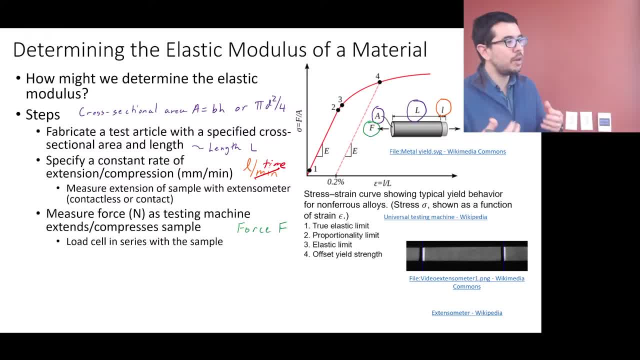 be some slop in either the gear train that's being used or in the hydraulics that are being used, but you don't have to worry about that, because you're going to be testing this machine. for a few seconds ago, The 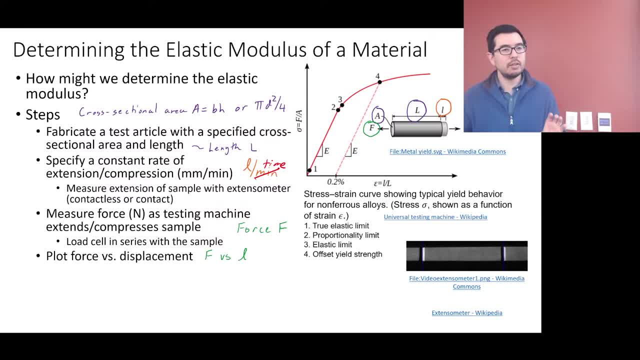 load cell is going to be in series with the sample, so it's going to be very fast and it's going to be very slow. So your sensors and everything else, it's our responsibility to convert these forces to stresses and these displacements. 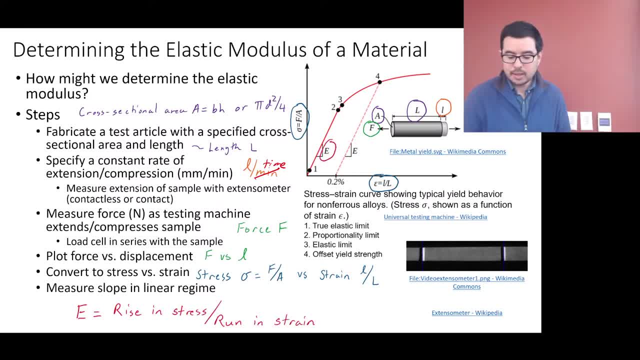 to strain. Sigma is equal to F over A N. strain is going to be the In the linear region, right? We said that sigma is equal to E times epsilon And that applies here. Any questions on this? So if someone gives you a strain curve, 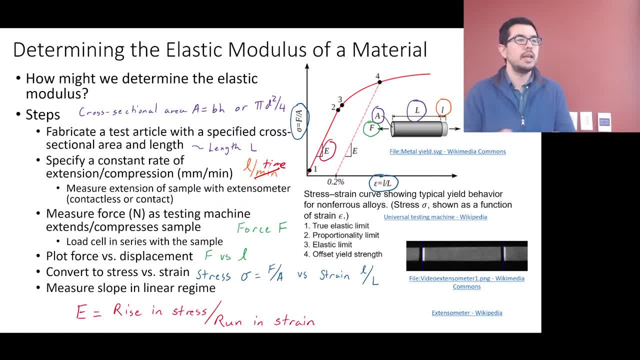 you have an idea of what they did to get it now And you can take out your handy-dandy ruler or you can do it by eye and you say, okay, I can figure out the elastic modulus Now if this graph starts at 0, 0,. 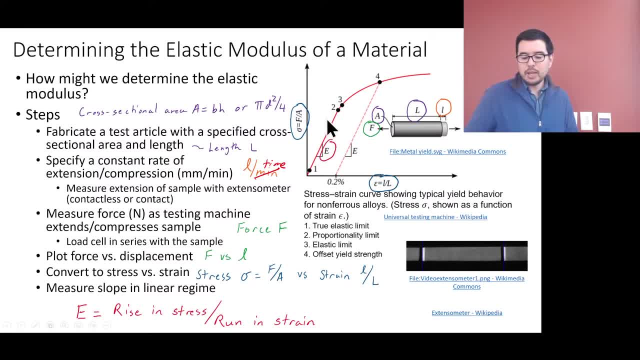 if the line's going through 0, 0, does it matter which point you pick? Not really right. As long as there's something below the line, The elastic limit or the proportionality limit, okay, Or these guys are even going farther. 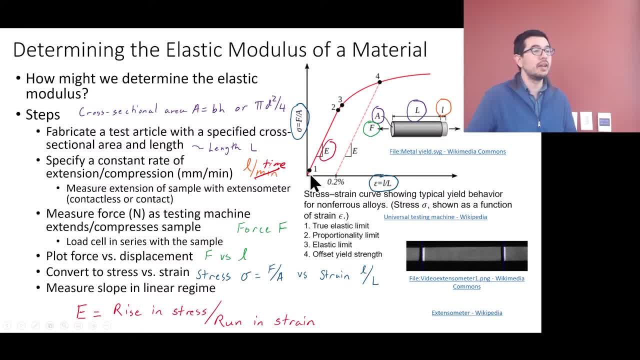 and saying that the true elastic limit is down here. But you'll see, like for some of the rubbery materials, you don't just trust what's going on really low. They actually will tell you this is the elastic modulus at 10% strain. 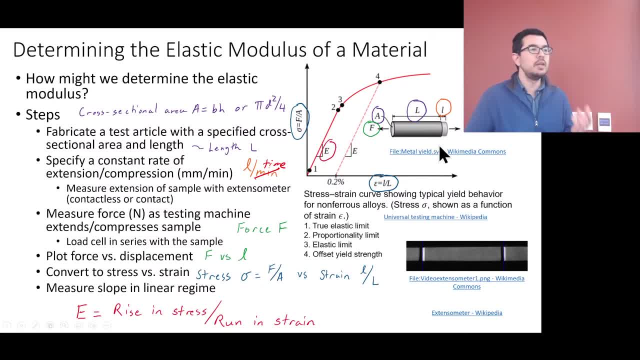 at a very high value, right? There's no way that a metal you're going to put a metal, a solid bar, I should say I mean a metal- can, of course, experience effective 10% strain if it's like coiled into a spring, okay. 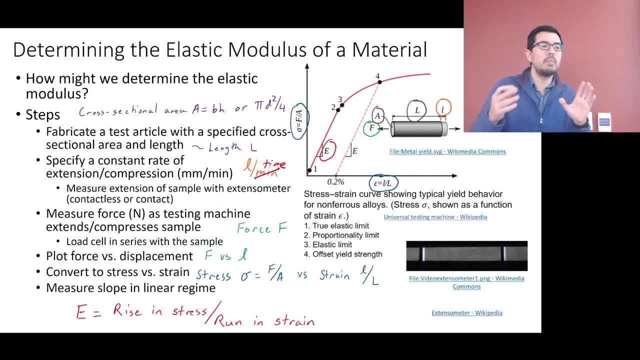 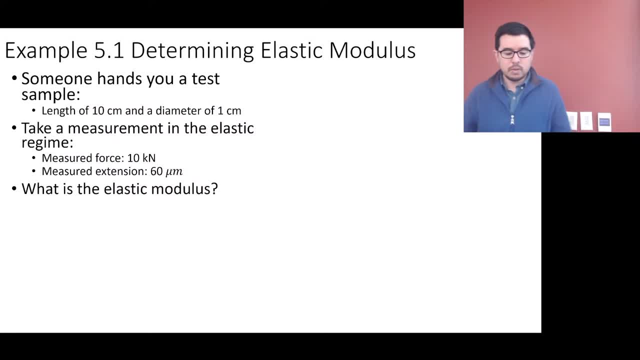 But there's no way that a bar is going to experience a metal bar. a solid bar is going to experience that and not have yielded Okay. so let's do an example. Someone hands you a test sample. The length is 10 centimeters. 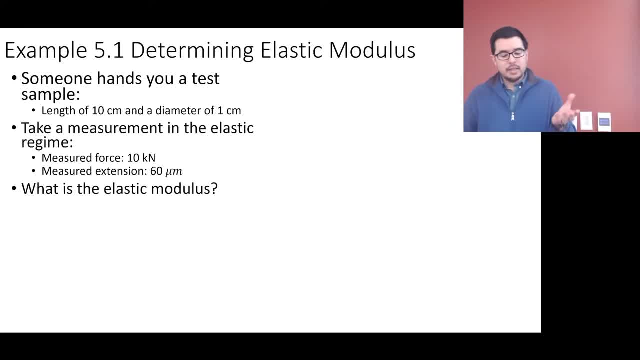 And the diameter is 1 centimeter. We take a measurement in the elastic regime and the measured force is 10 kilonewtons. The measured extension is 60 microns. What is the elastic modulus? okay, So we didn't have to build the machine. 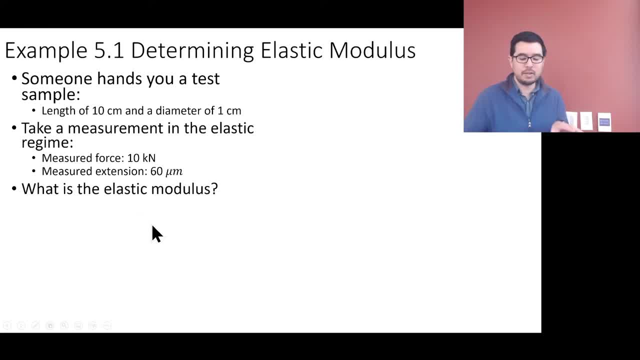 and do all those details, work out all those details right. We just have a few numbers that we need to calculate the elastic modulus, So let's start with. well, why don't I calculate the stress right? So sigma equals E. 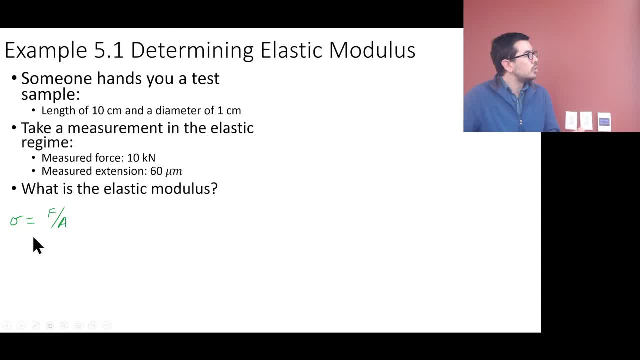 sigma equals E- epsilon. okay, So they told us what a force was in the elastic regime. They told us that the diameter was 1 centimeter, right, So we can calculate out. force divided by area: Sigma equals E- epsilon. How many times are we going to say this? 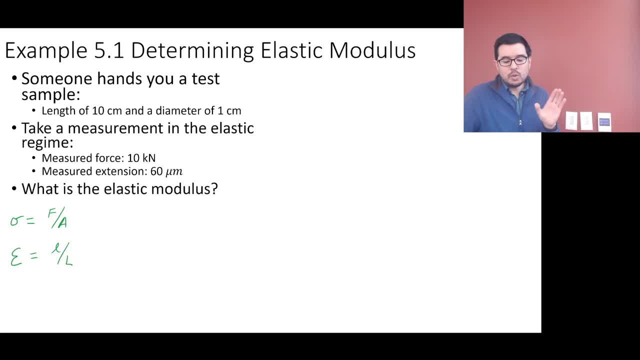 A lot of times this semester. okay, So how do we calculate out epsilon? Epsilon is the length that we've had in extension, So that's 60 microns divided by the initial length, That's the 10 centimeters. okay. 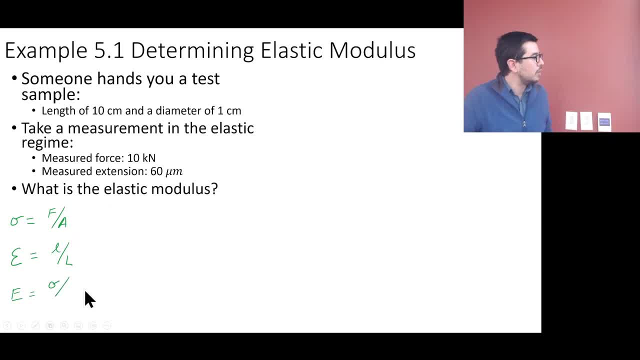 So we can figure out what the epsilon is. So E is equal to sigma over epsilon. right Sigma was equal to E. E is equal to E- epsilon. So we need to figure out what E is equal to. So we go through this. 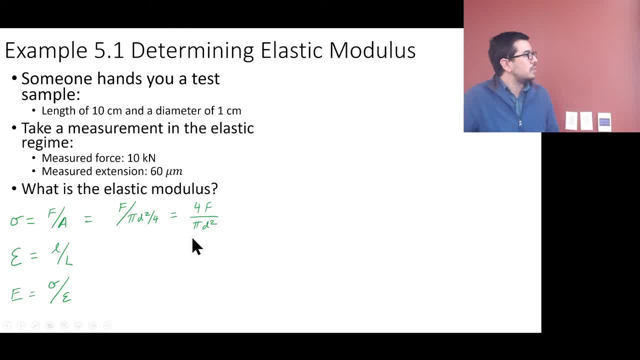 Area is pi D squared over 4.. It comes out to be this The end result. right, So we had. this is the epsilon going right into here. right, This is the sigma going right into here, and this is what you get. 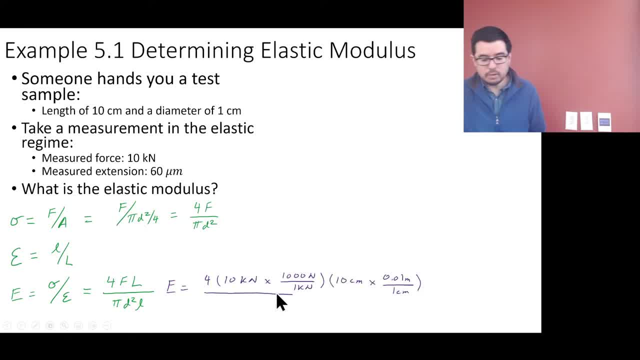 And then if you write it all out and you're careful with the dimensional analysis, which I understand, it's frustrating, okay, And it takes a little bit of space. okay, But 10 kilonewtons is, you know, 1,000 or 10,000 newtons? 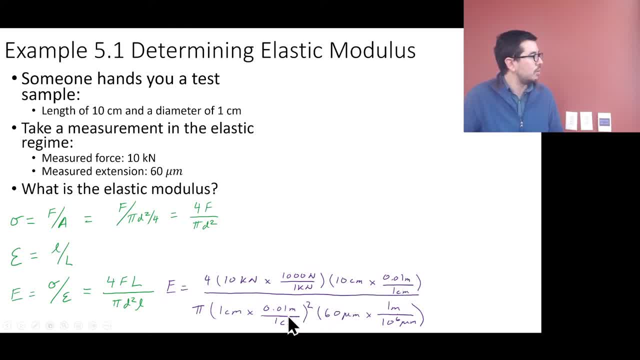 Centimeter right is 0.01 meters, All these things and like: if you have a square, sometimes it's easier to keep it in the square. So do the one centimeter right, Do that conversion inside and then square the whole thing. 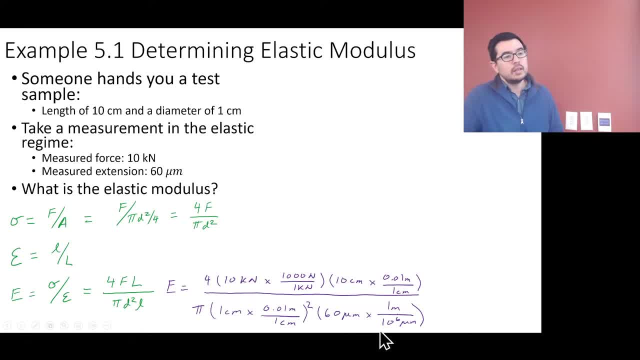 A micron right is 1, 10 to the minus 6 meters. all right, So that's these things. And then also, typically what you're looking at is the elastic modulus given in gigapascals. So first we converted everything to newtons per meter squared. 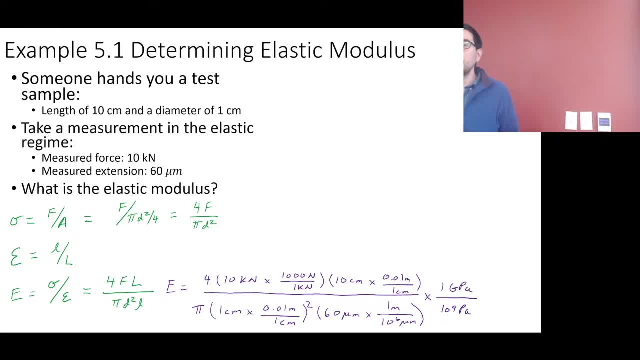 and then we're going to essentially multiply by 1E or 10 to the minus 9, or divide by 10 to the minus 9 to get it in gigapascals. So when we do that, we get about 212 gigapascals. 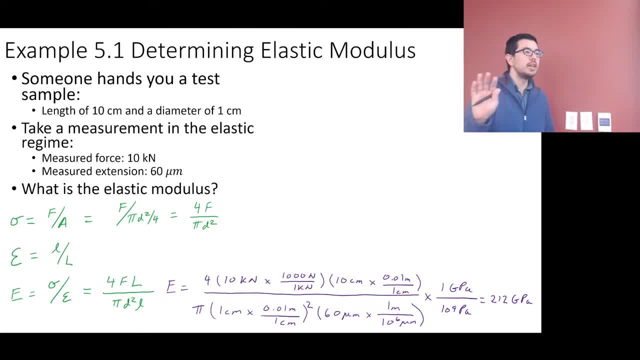 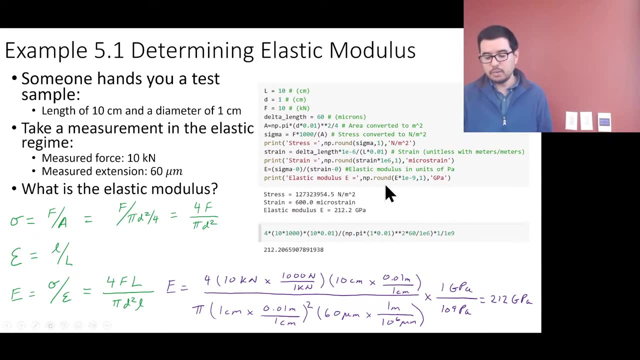 Any questions on that? Nice, straightforward, okay, And if you want, you can look on the IPython code that's included with it. You can go to the session and you get that result. So what I did I did at first. this is like code speak. 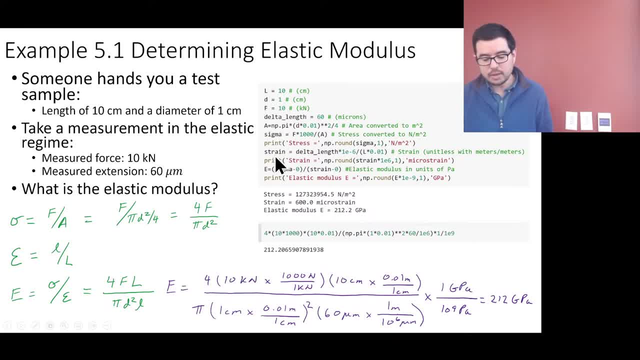 right, kind of like: okay, I'm first going to calculate out sigma, going to calculate out strain, and then I'm just going to do sigma divided by strain, right. But if you want to just jump right to the whole shebang, 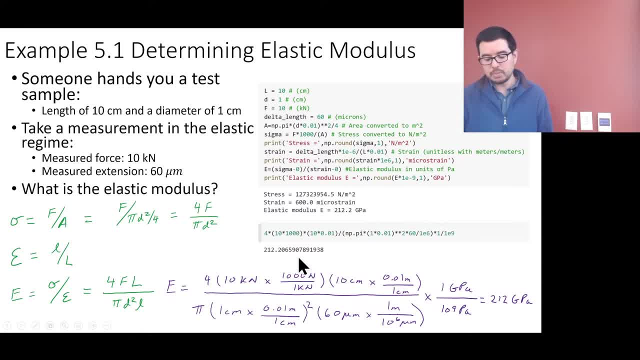 right, you write this out on your formula sheet or on your piece of paper, then you can just use IPython as a calculator, It doesn't matter, right Either way, But this lacks the variables, okay, So it's not as convenient as just being able. 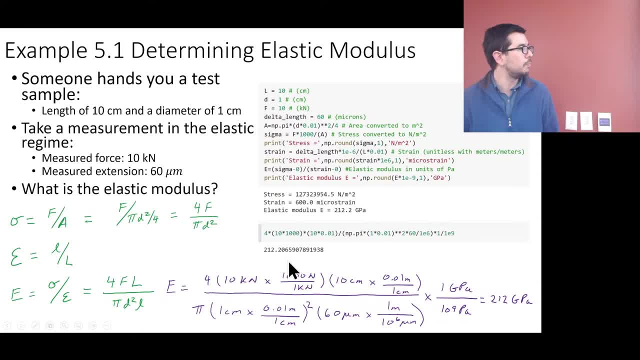 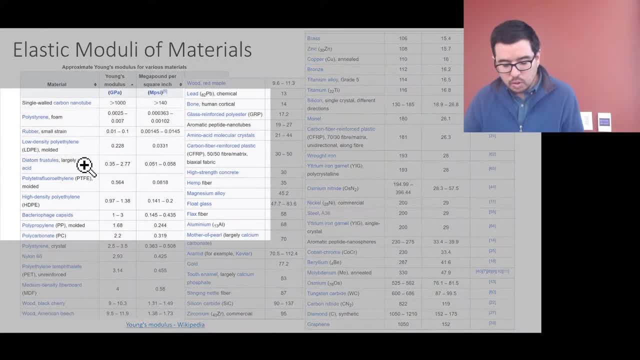 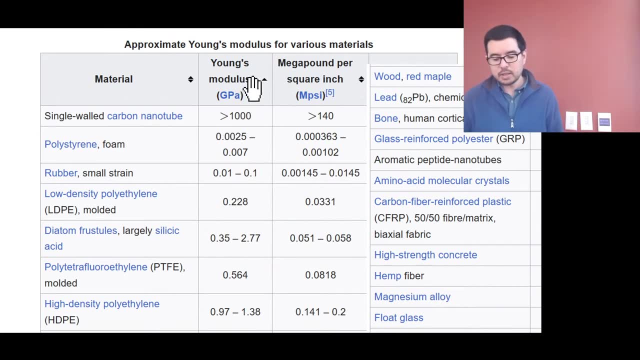 to change the variables, the values here, and be able to change them. Okay. so look at this chart. This is craziness but it's fun, okay, So these are materials: Young's moduli and gigapascals. 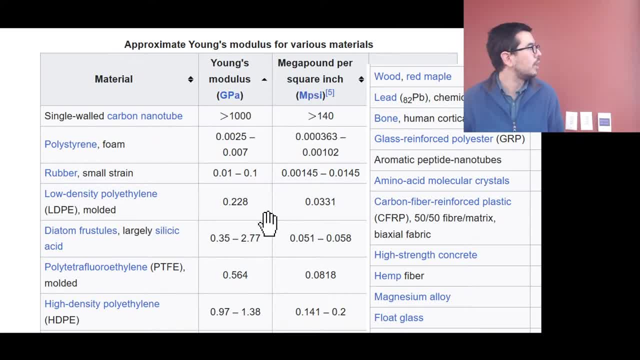 Okay And they're sorted, except for this one because it has greater than okay, which I guess means it gets down at the very bottom. They're sorted from. they're in ascending order, All right, and you can look at the webpage. 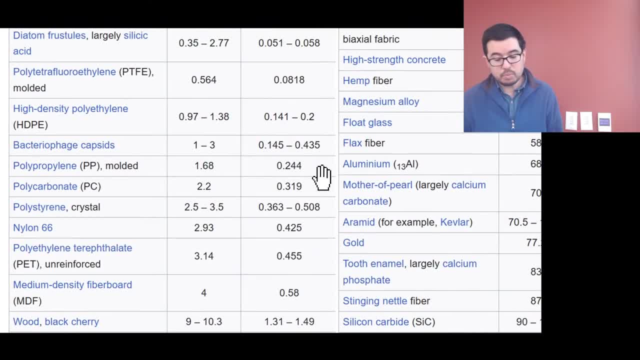 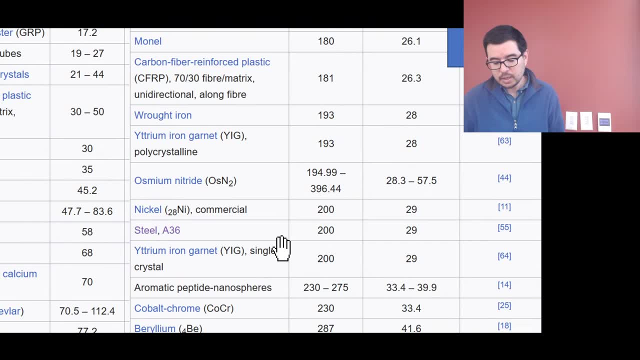 This is a Wikipedia page and, from what I can tell, these numbers look pretty reasonable and pretty accurate. Okay, So here is steel. This is a 200 gigapascals. okay, 210, 200.. That's what I would use for steel. 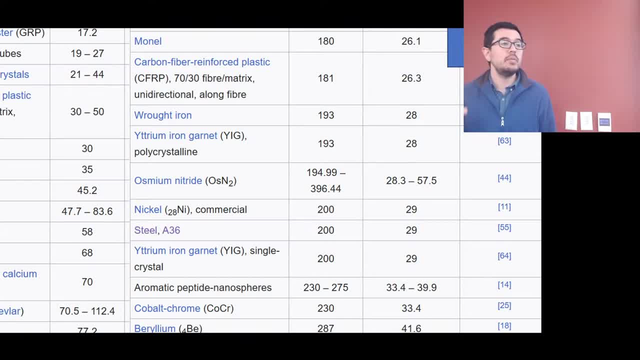 One of the interesting things about steel is, even when you alloy it so you have iron and carbon and some other stuff in it, they pretty much all have the same elastic modulus, So strength could change quite a bit Quite drastically. In fact we talked about that last time. 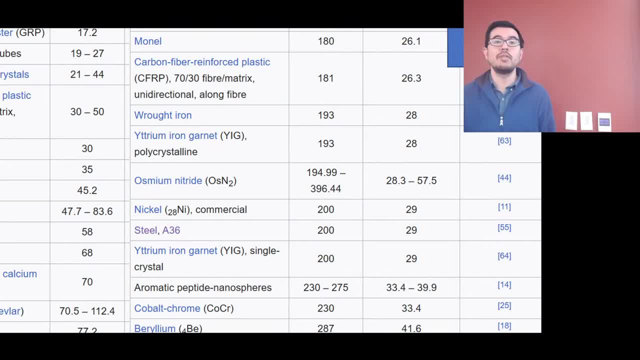 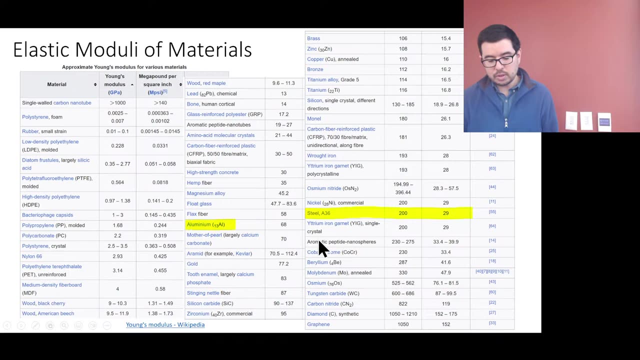 And we said it could go like from 10 to 700 megapascals or strength. Okay, but the elastic modulus is gonna stay the same If you break this down. I highlighted some of the ones that I think are kind of good to know. 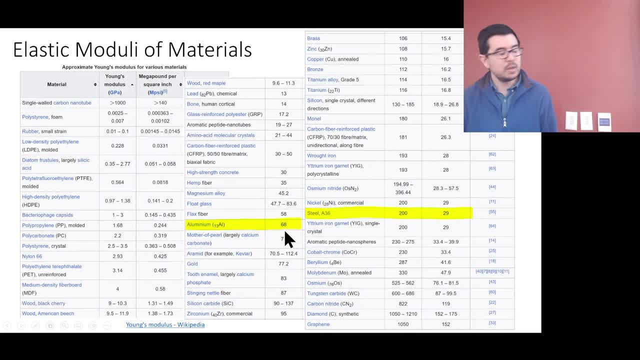 Steel at 200 gigapascals, Aluminum at about 70. You can't see that that's a 68 titanium. okay, yeah, there might be some problems. that's around 120, 116 is what that is. gigapascals would around 10 gigapascals and then the 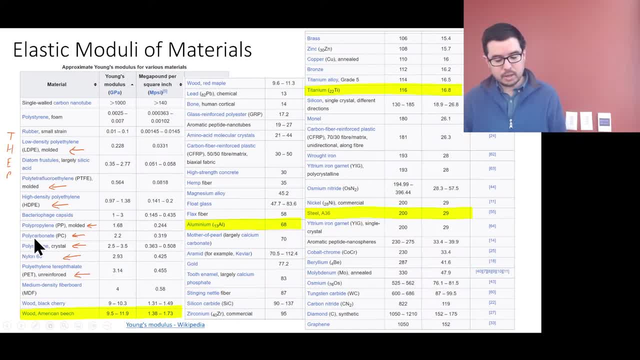 thermoplastics okay, which are being highlighted here. you can say that they're on the order of a gigapascal okay. so you've got. you've got a lot of range for the elastic moduli, but it's only. it's only three orders of magnitude, or two orders of magnitude, really. actually, you get less you can get. 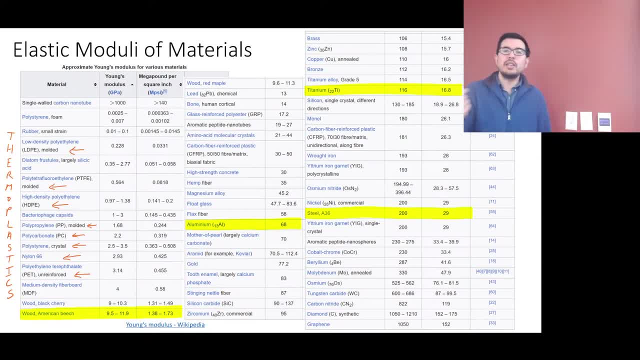 less than one gigapascal, okay, but if I give you a resistor, right, I just pull out the resistor in my kit. I'm like, oh, is this mega ohm or is this like one ohm? that's six orders of magnitude that the electrical engineers have okay for. 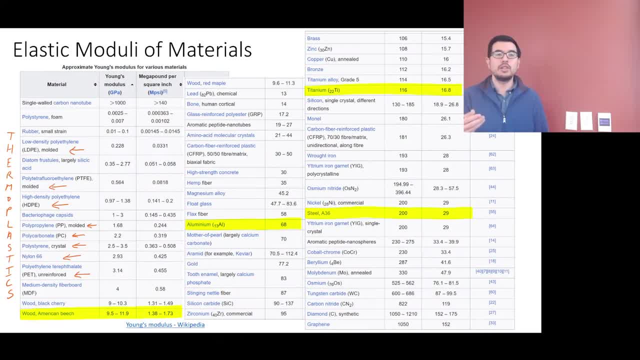 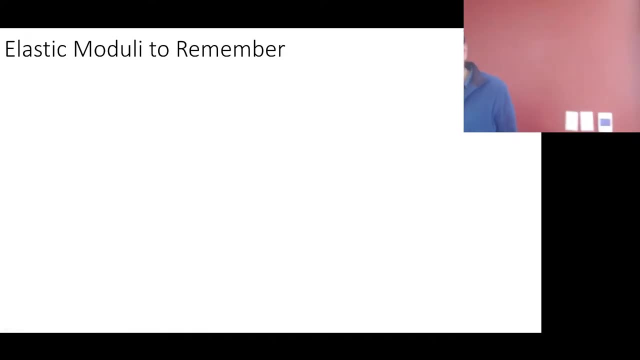 elastic moduli and stiffness. we don't have that much variability and the materials are. it can be quite different. oh yeah, and the rubbery materials which I like. that is 0.01 to 0.1 gigapascals. so these are some of the elastic moduli. to remember, steel, around 200 to 210. 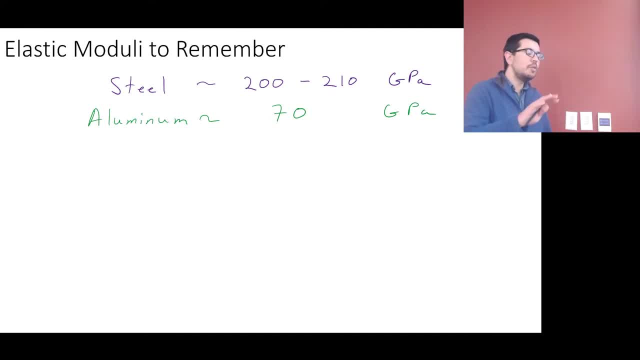 gigapascals. I made an agreement so if you look, don't worry. on last semester we wanted to hit on the final, so I said okay, on the final, question 1a will be: what is the elastic modulus of aluminum? all right, I just told them. all right. they got a point. okay, 70 gigapascals. the typical rule of thumb is that steel's elastin, the elastic modulus of steel, is three times that of aluminum. that's just the rule of thumb, okay, but I guess you could just remember both of them it. 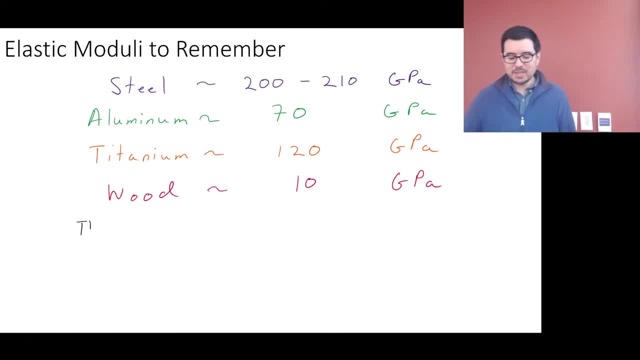 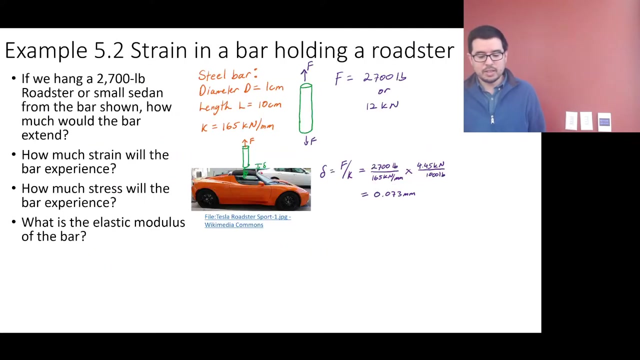 doesn't really matter. okay. titanium, like we said, 120 wood around 10, thermoplastics around one and rubbers a fraction of that in gigapascals. ten minute ten to the nine. one giga pal, get one gigapascal is a thousand megapascals, okay. so these are some to remember. now let's go back to that. 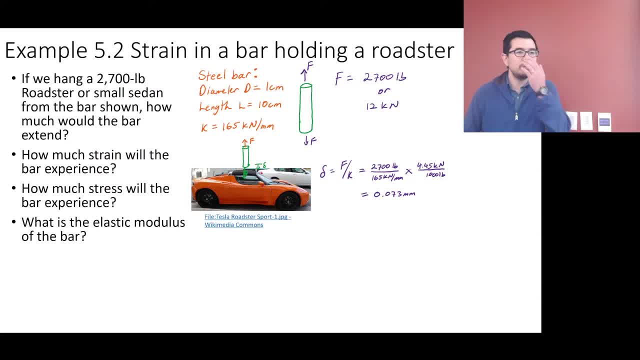 example we did- I think this was the second. yeah, as a second time we met where we said: I'm maybe it's the third time. no, it's the third time because we did bars of springs. yes, the third time. so here's a 2,700 pound force pulling this bar apart. 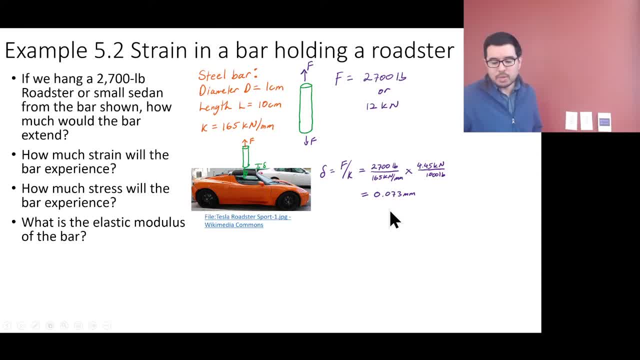 and we said that it had a little bit of deflection: 73 microns. okay, now let's ask ourselves some other questions. how much strain will the bar experience? how much stress will the bar experience? what is the elastic modulus of the bar? okay, so strain, that's gonna be essentially how much displacement we have over the 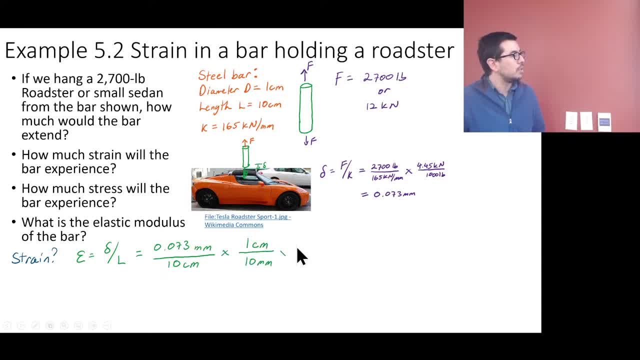 initial length, so we can do this all out, right. that's the 73 microns, and we said that the length of the bar was ten centimeters even back then, so the strain ends up being 0.07 3% stress. well, that's going to be force divided by area. 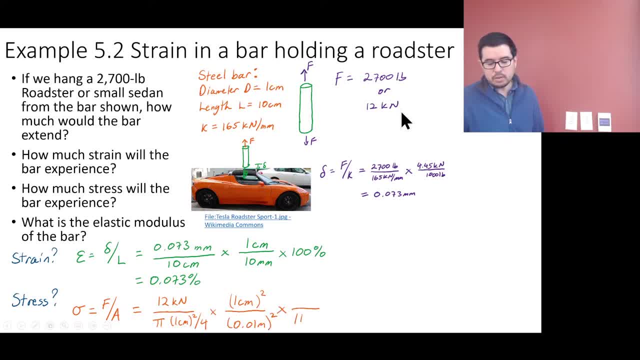 So we have 12 kilonewtons of force. take the area as being pi d squared over 4, and we make sure we convert appropriately. We get all into newtons per meter squared and then we multiply by 10 to the 6th, or divide by sorry, divide by 10 to the 6th to get in megapascals. 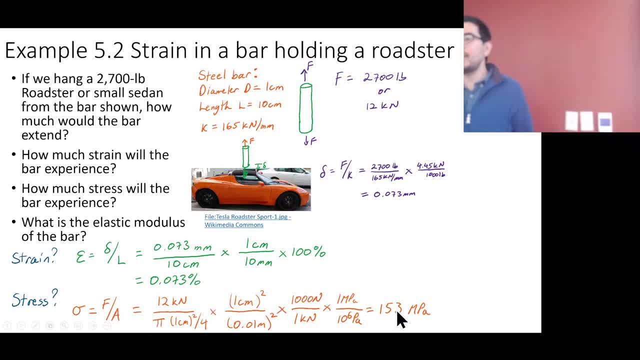 So elastic moduli are often in gigapascals- right, you're starting to see this because you have, but then we have these really small strains. like this is representative value. this is. you know, this is for some steels that will break some steels- okay, 153, but that's not unreasonable to find a steel that has a yield strength greater than 150 megapascals. 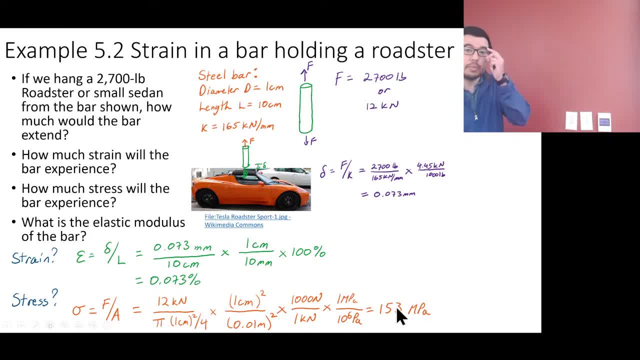 So, yeah, what I was saying is the stresses are often in megapascals And elastic moduli are often in gigapascals. So elastic modulus right is going to be given by sigma over epsilon, and so we've now calculated out epsilon right here, calculated out sigma and we get 210 gigapascals. 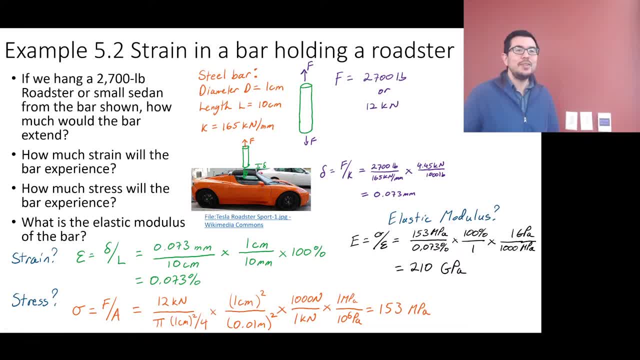 Is that a coincidence? No, I tried. I tried. I'm not perfect, but I tried to design the problem to use the elastic modulus. I tried to design the problem to use a realistic k- okay, So now let's ask the question. wait, we have these k's, this is Hooke's law, but we now have another form of Hooke's law. 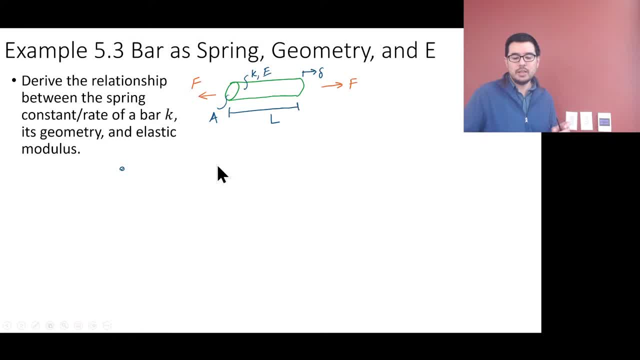 How do we relate geometry, elastic modulus and the bar to each other? So you remember we spent a whole time, a whole session, looking at this is the k-phi, This is the bar, And people are like: where did this k value come from? 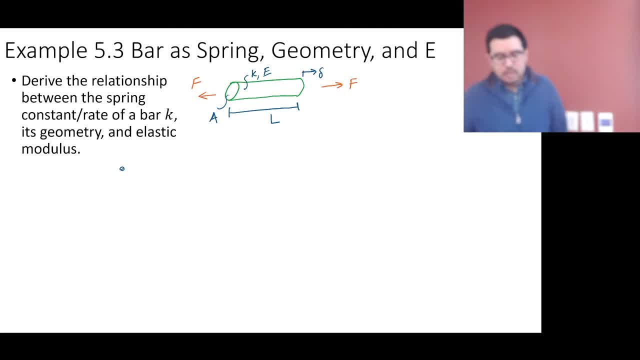 We're about to show you. It comes right here We have Hooke's law. Oh, I guess we should maybe say that: all right, there's a k, there's an e right. So k was what we said in terms of kilonewtons per millimeter, right? 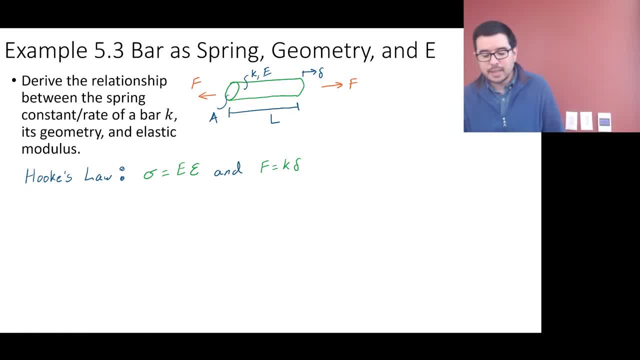 That's the spring. constant force equals k delta. E is the elastic modulus. Delta. Delta is how much this bar extends. L is its length, initial length, And f is the force Area. is the cross-sectional area Or a is the cross-sectional area? 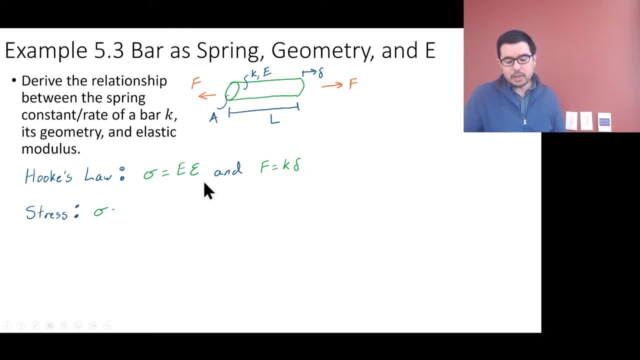 Okay, so the two forms of Hooke's law are: sigma equals e epsilon and f equals k delta. The stress is just: sigma equals f over a. The strain is going to be the delta over the l. So let's essentially just do some algebra and combine some things with each other. 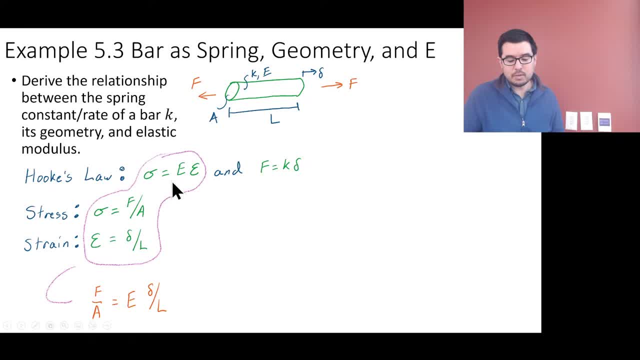 So here we can write a new expression, right where we have sigma: is equal to e, epsilon. So plug in f over a on this side And plug in epsilon, which is right here, the delta over l, And now we have the e. 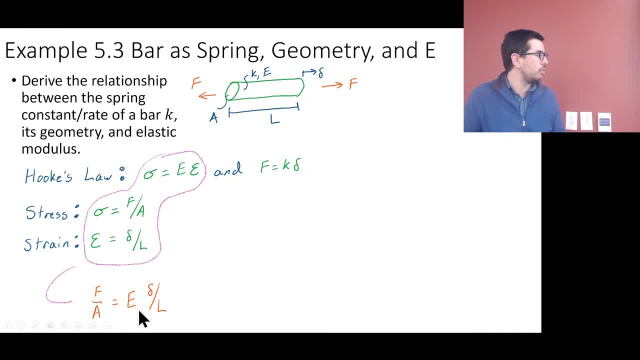 Let's say we, you know, one of our goals could be to try to solve for the e. Or maybe our goal is to solve for a k. Okay, let's do looking at e here All right, and then drop it over into figuring out what's happening with the k. 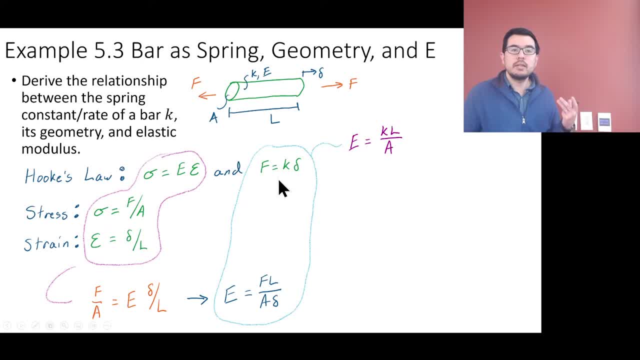 All right because, remember, we had this idea of a something newtons per meter for a spring constant, So we put these in here, right? So we have, e we see that, oh, I've got this l over delta. 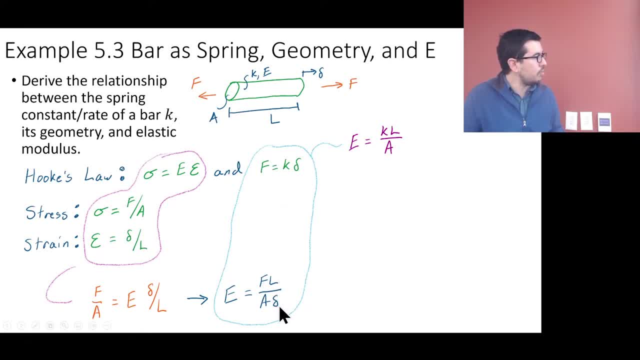 That, or I've got this sorry f over delta, right, And I've got an f and a delta, And so now I can pop in a k here. So e equals kl over a, And we rearrange things. 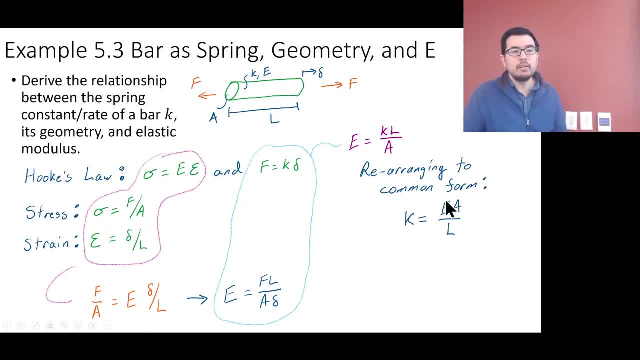 And we get that k is equal to ea over l. This is one to write down. Now, what does this tell us? right? We like to think about scaling. This is not. This is not. This is not the scaling relationship that we had. for how much load can a bar support? okay? 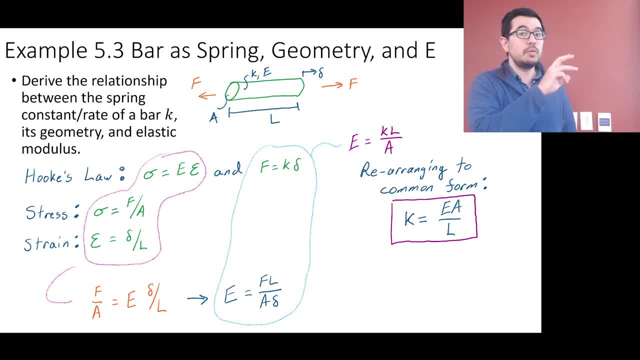 We can do that one real quickly now. actually because we know that sigma is equal to f over a. All right, do you remember that? So sigma is equal to f over a and we say: hey, there are yield strengths. 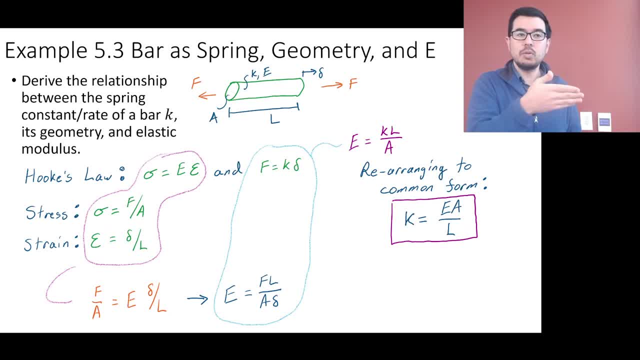 There are maximum yields or maximum stresses you can get to. So constant equals Force divided by area right. And we said, hey, the supportable load that this bar can support is proportional to the area right. So if I increase the area, I can support more force. 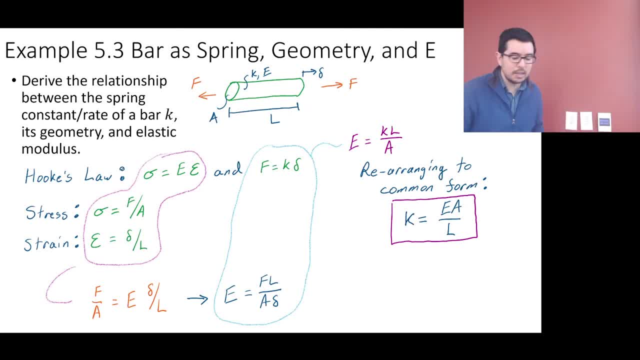 Okay, that's the stress Here. what we're talking about is stiffness, right? So how much displacement do we get when we apply a given load, all right. Or how much force do we get? right? Probably better said, because it's k delta. 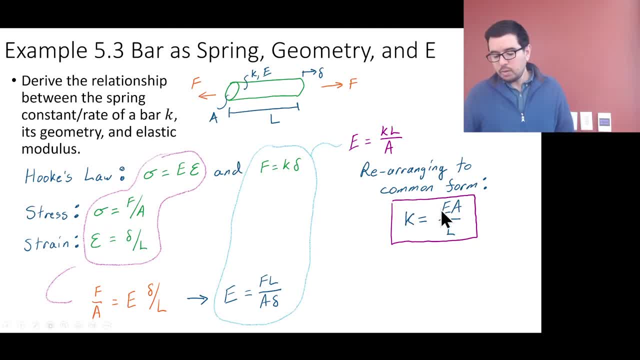 So look, if you use a material that has a higher elastic modulus, you have a stiffer bar. If we increase the cross-sectional area, we have a stiffer bar. And then you remember: springs in series. what happens? Well, you get decreases in the k's. 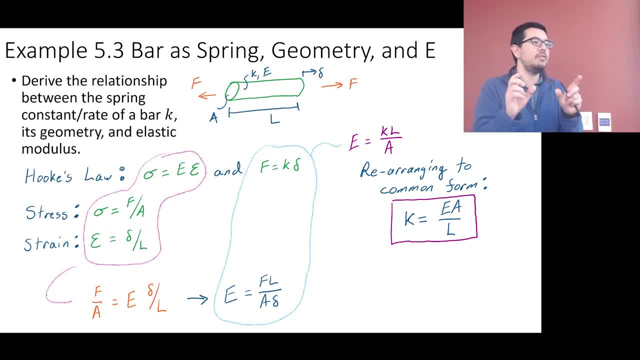 Remember we said if you double The length of the spring, you're going to half the elastic constant or the spring rate, the spring constant. okay, So now we have a relationship based on what we know from Hooke's Law and it has two forms and stress and strain. 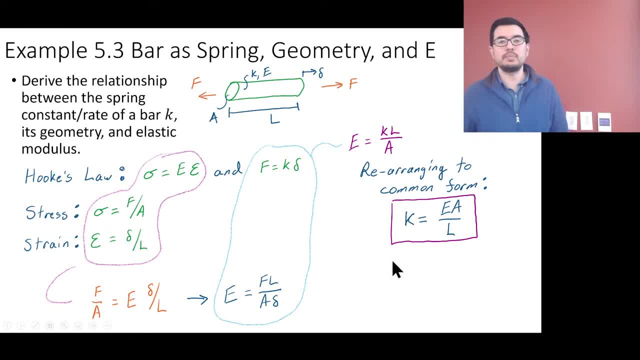 So we can calculate what the k's are. So it's no longer a mystery. Now, if I have an indeterminate problem, is it easier or harder right to think, oh, I have this. I have Essentially three more terms. 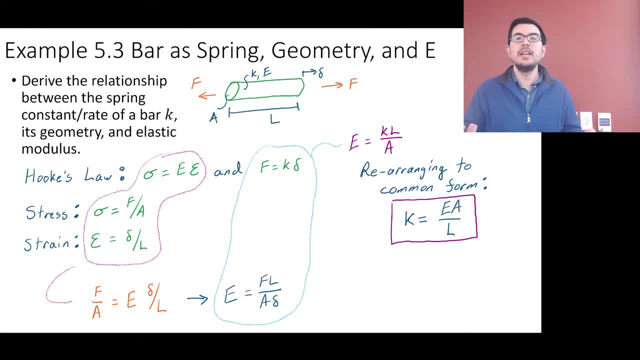 I have ea over l or I just think in terms of k's and stiffnesses. I think in many cases it's easier to think in terms of the k's. Okay, so you do the problem in k's and then eventually you can plug in ea over l or figure it out, depending on what you need to figure out. 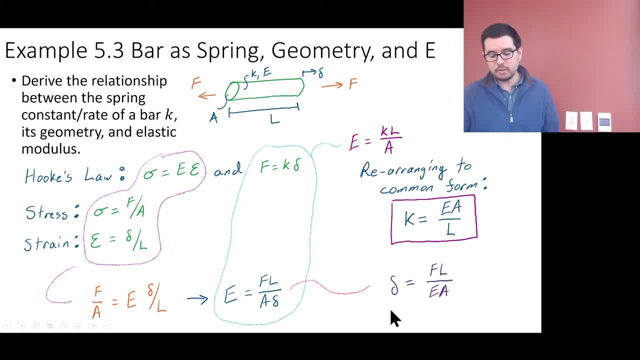 Now another relationship. this is also to be written on your formula sheet, and this is a famous one: Delta is equal to flea okay, Or I often say flea Okay, Or I often say flea Okay. pl over ea. 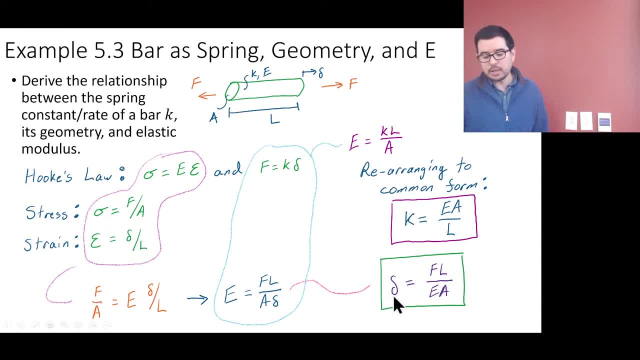 So this is a relationship that tells us how much stretch right, how much change in length we're going to have, how much extension we're going to have for a given amount of force. If I increase the force, I get more extension. 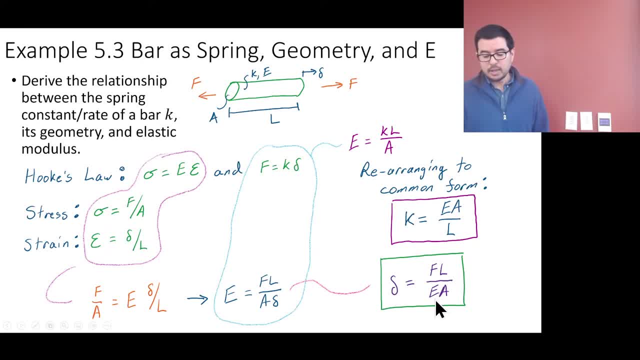 If I increase the length, I get more extension. If I increase the elastic modulus, I get less extension. If I increase the cross-sectional area, I get less extension. Okay, Again, these are all kind of intuitive scaling relationships that we've discussed in some way, I guess, when we were talking about springs and series and parallel. 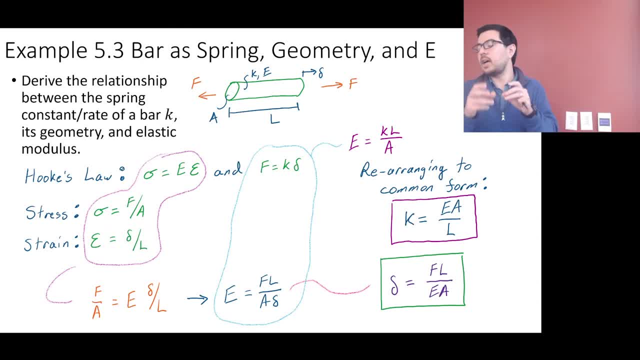 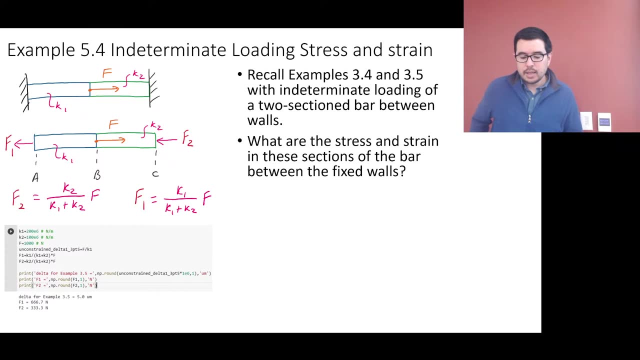 But now we have concrete equations that allow us to think about what those values would be for a bar. Any questions? Okay, So let's look. Let's look at an example with indeterminate loading. Okay, This is the same one. 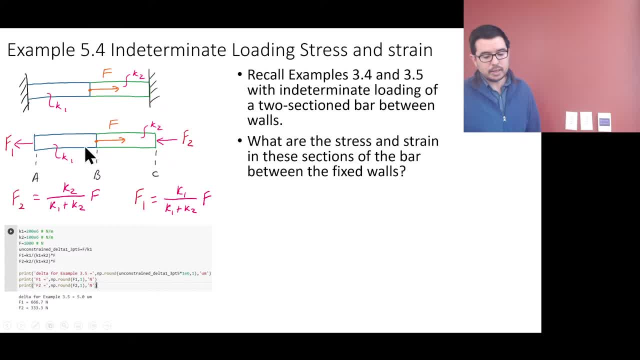 This was back from session three, okay, where we were using the k's And we said, hey, the internal load in this member is proportional to the stiffness in that member. So if this is a very stiff member, that means that this internal load is going to be quite high. 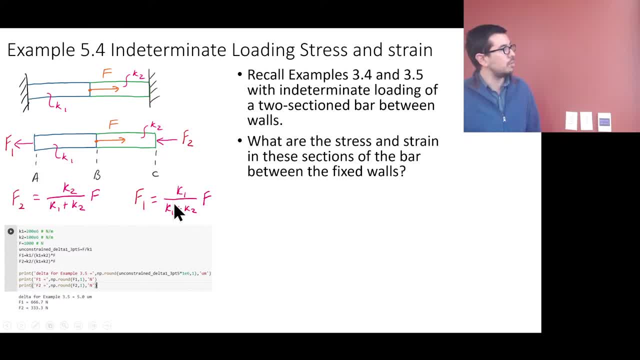 Okay, So we get k1 over k1 plus k2.. This ratio would be close to one, And it's close to what this force is being applied in the middle. Okay, And the same thing was true for this force here. 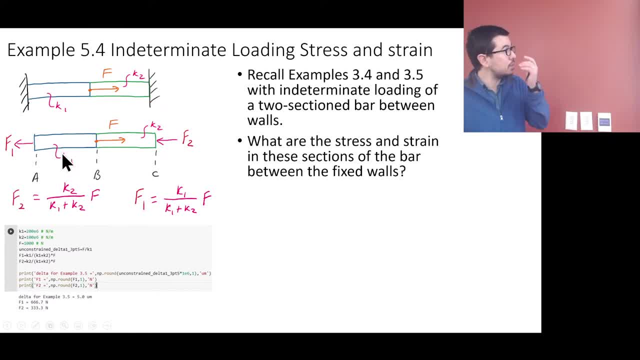 Notice: these arrows are in opposite direction. This opposite direction, This region is in tension or compression, assuming f is positive, Tension right. And then this region right is in compression, It's being compressed. So these signs are all correct for the forces. 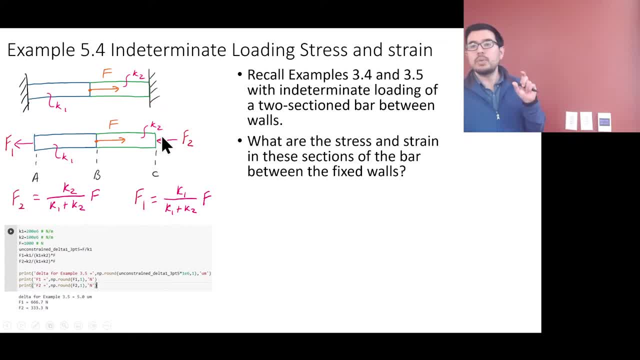 They're both positive forces, but they are in opposite. They're doing opposite things: The behaviors, the materials experiencing compression in one case and tension in the other. So if we want stress and strain in these sections of the bar, between the fixed walls, 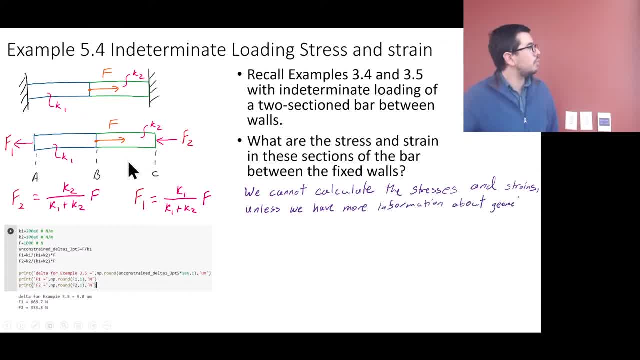 we can't do it unless we have a little bit more information. Okay, Like I can't tell you, if you don't tell me what the cross-sectional area is here, I can't tell you what the stress is going to be. 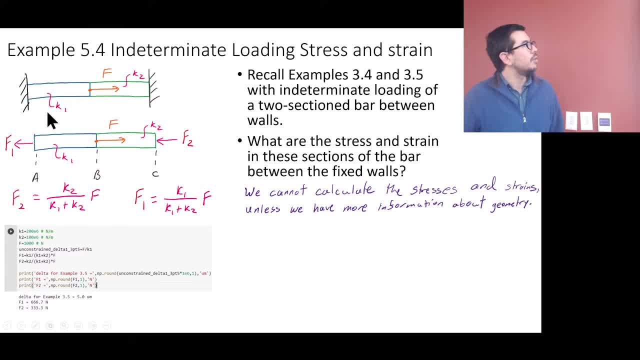 But if I told you the length, alright, and I told you what the material was, alright. so if I know the length of this section and I know the resulting, and I know the resulting delta, Because I know the elastic modulus and I know that length and I know that strain, 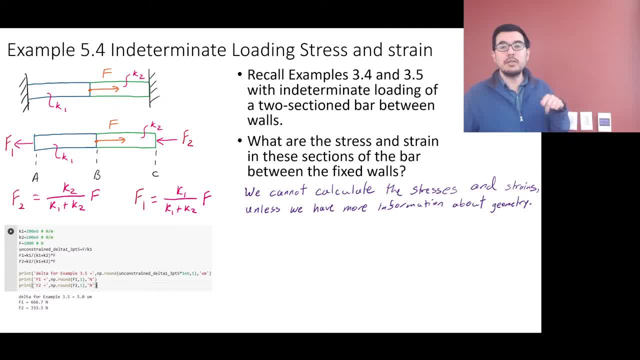 and I can then relate it to stress, because I know that sigma is equal to E, epsilon, right? I don't know how many times I've said it, but that gets said again. Okay, so let's say: what are we going to give us? 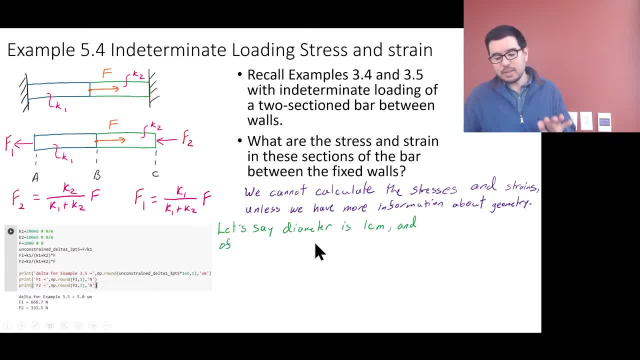 What are we going to work with? Let's say that we're given the diameter, okay, And let's say that the material for both sections is 2.5. Okay, Okay, And the material for both sections is 200, is steel with an elastic modulus of 200 gigapascals. 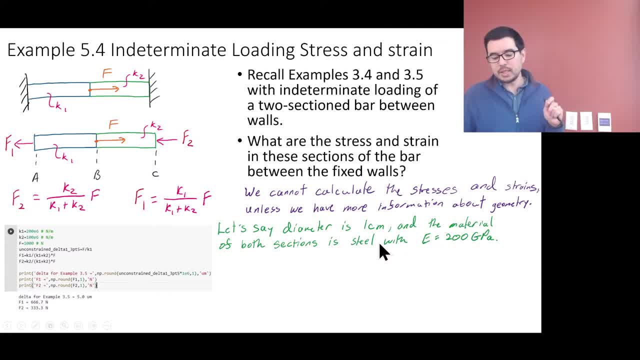 Okay, so now we have a little bit more information. we have something about the geometry. right Before, we had essentially nothing besides that there were Ks here and that these were between two walls. We didn't know their length, we didn't know their cross-sectional area and we didn't 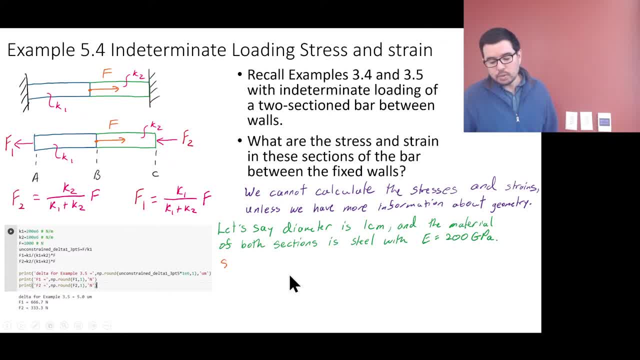 know the material either. So if we know the, The, The, The Diameter right, We can figure out what the cross-sectional area is and we can figure out what the stress is. So this is taking F over A right. 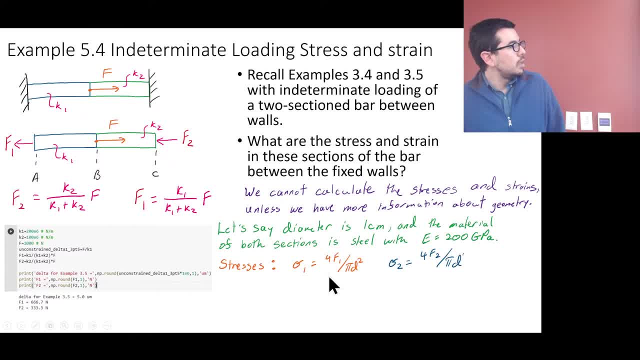 Pi D squared over four. Now, did I do this right or did I make a boo-boo? Sigma two is equal to four, F2 over Pi D squared. This is where we should be careful. we might want to put a negative there. we do want to put a negative, because that's a compressive. 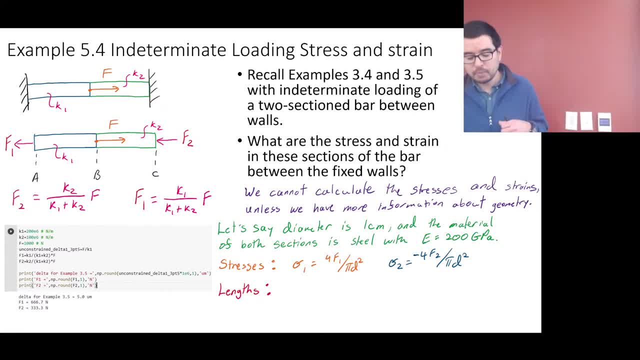 stress, our lengths can be calculated from using our formula. right, we said that K is EA over L, so now we can say that L is EA over K, so we can calculate the initial lengths. and because they told us what the K's, I told, well, we were given K's right there here, 200 kilonewtons per millimeter. 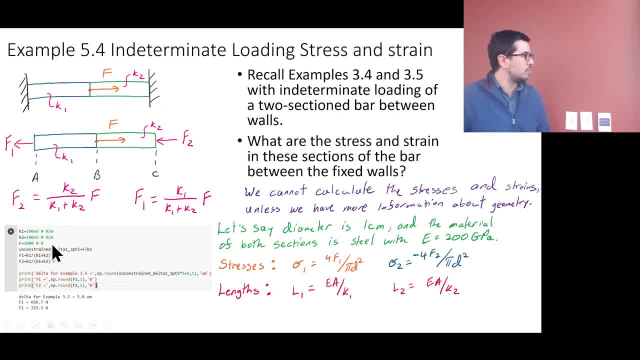 or 200 times 10, to the 6 newtons per meter. that's really small, and so we can figure out the initial lengths. we can also figure out the strains, and strain can come from hooks. law in terms of Sigma is equal to E, epsilon, okay. or in this case, epsilon is equal to Sigma over E. and should I be careful? yes, I should be. 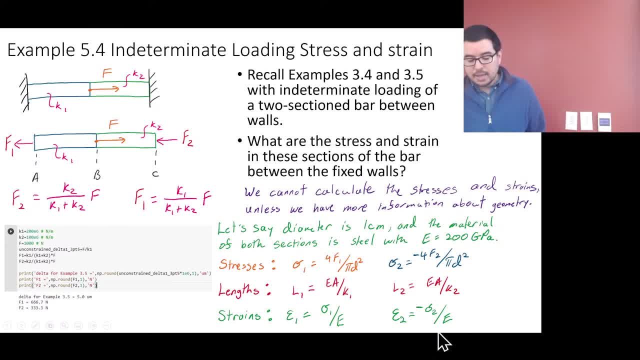 careful and add a negative and here, or I mean this is a little bit tricky- because if Sigma 2 is negative, All right. So I actually I mean, I, I might take this one out here, Okay, And this is where kind of having a sense, right, Because if sigma 2 is negative, that means that the strain is going. 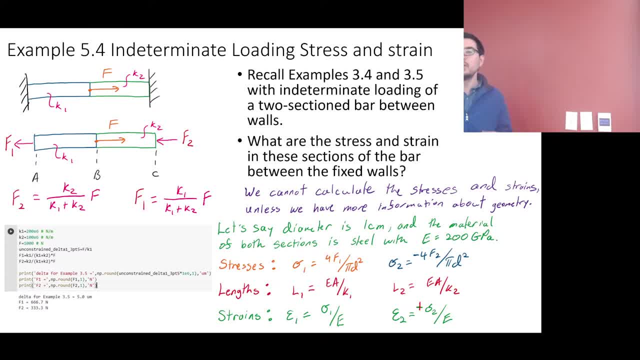 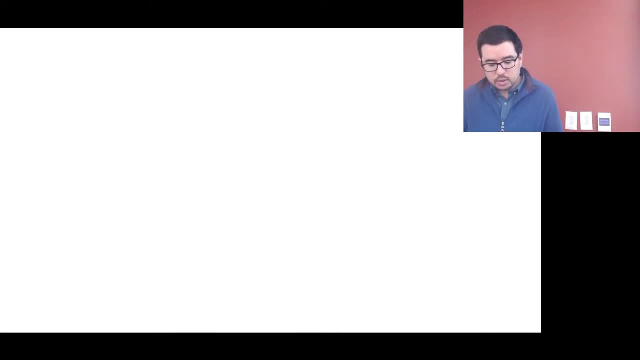 to end up being negative automatically, Okay. So sometimes, when you do these problems, you'd be like: is it going to be negative or positive? Okay, And sometimes it depends on which way you're defining the errors. Okay, Coming out of it, Okay. So that's, that's how we go about solving. 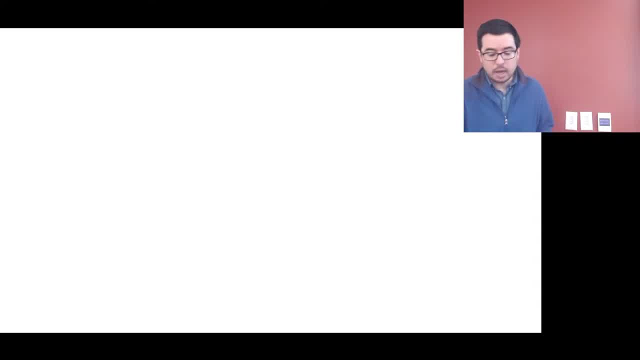 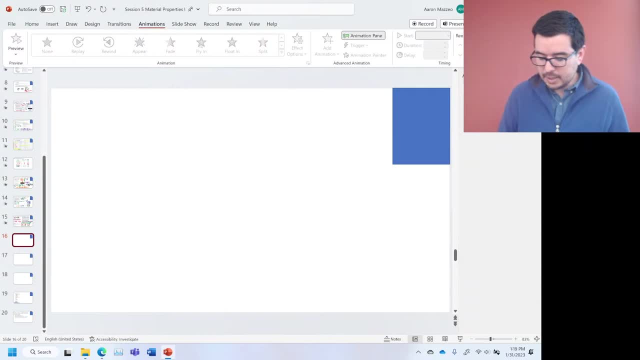 those All right. How much time do I have? I don't have much time I wanted to do. I just wanted to do a couple of things. Okay, Yes, Okay, Let's, let's do this and then we'll we'll talk about. 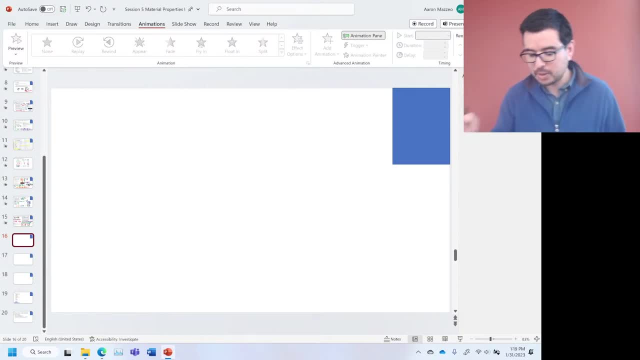 something else the next time. No, let's, let's do this and then we'll talk about something else next time. All right, So okay, Those are axes for a stress-strain curve. This is a stress-strain response. Okay, Let's say that I don't know. this value up here is a hundred megapascals. Let's say this: 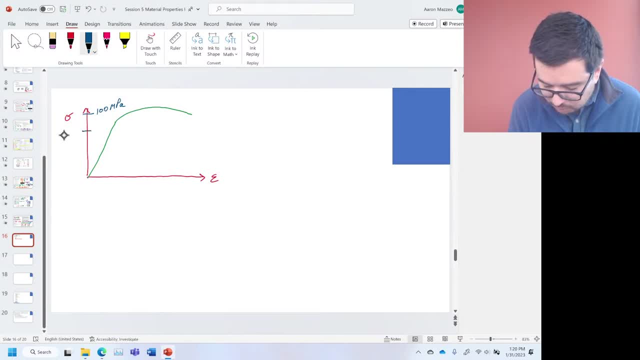 value down here is like 75 megapascals. All right, So like this is kind of coming across like there. Okay, So let's say that this value right here is 0.1%. I'm going to copy this because I want to do a couple of different things. 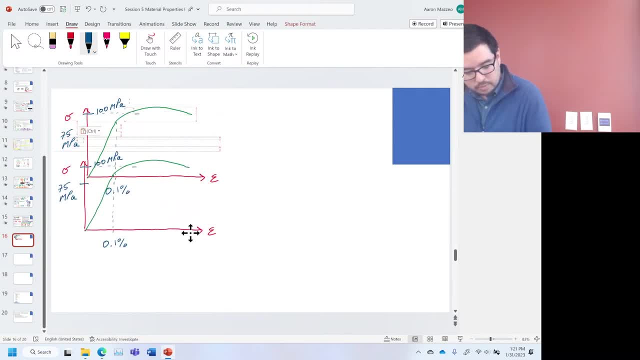 Now, if we get rid of thisyl gamma, you can do this, even if it's a least Okay. So in the first case, let's say that we load past sigma y. All right, Sigma y is here, All right. let's just say I don't know what it is. 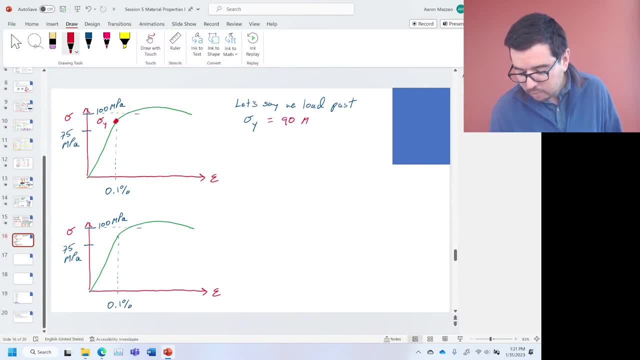 Let's say sigma y is equal to 90 megapascals. So we go up, we go up, we go up. Let's say that we actually get. we get all the way and we get to 100 megapascals. 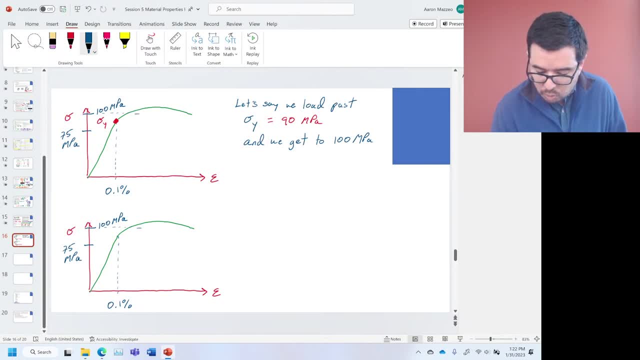 All right. so we end up getting all the way up to this point, right here. If I had stayed below the proportional limit, below the elastic limit, all right. if I had stayed in this region, I would have just gone right back down. okay to zero, zero. 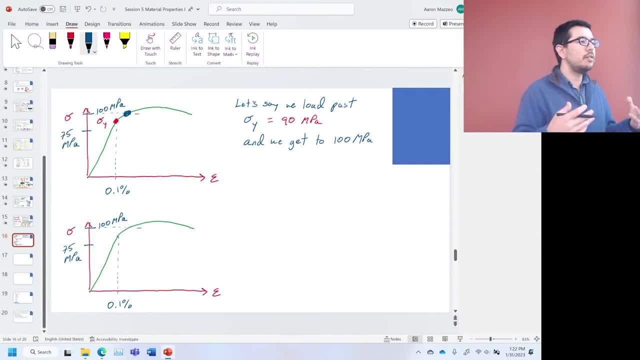 Okay, would have sprung back, No problem. No problem, right? If I'm a muscle or something, you know, I'm just like I am just doing this over and over again. So let's say that, like my buddy decides that I can handle a little bit more weight, right? 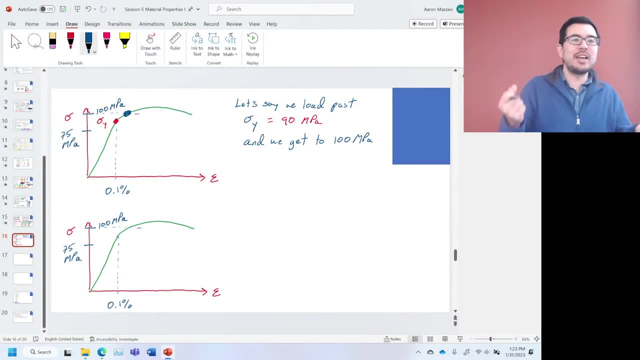 And I get pushed to have more stress applied to my muscles. okay, So then I get up to this level And it hurts. It hurts. And what happens when I drop the weight? Do I get to spring back to zero, zero? 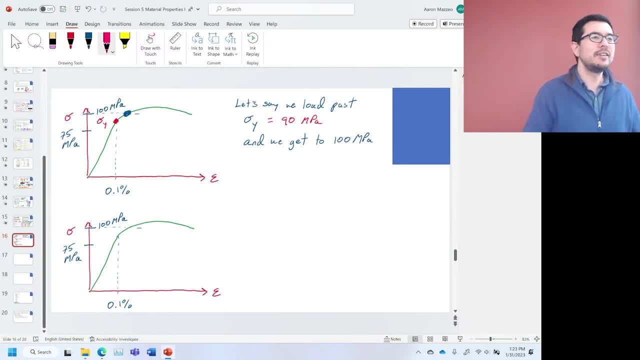 I don't, But where do I go? Where do you go right? Well, for the materials we're dealing with, what we assume is that the slope right. remember, this is a, This is a. This is a. 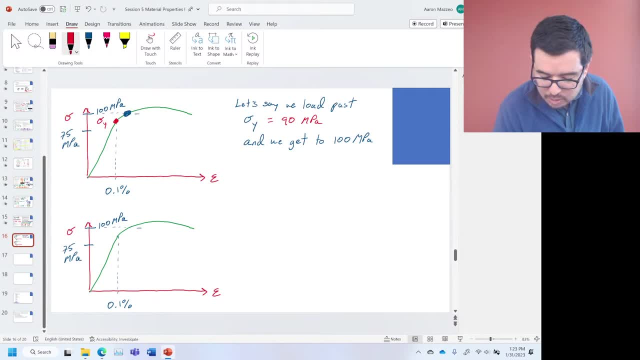 This has a slope of E. here You follow the same slope. I want to use a color that. Ah, that's a good color. We're going to follow the same slope back down, okay, And this is referred to as residual. 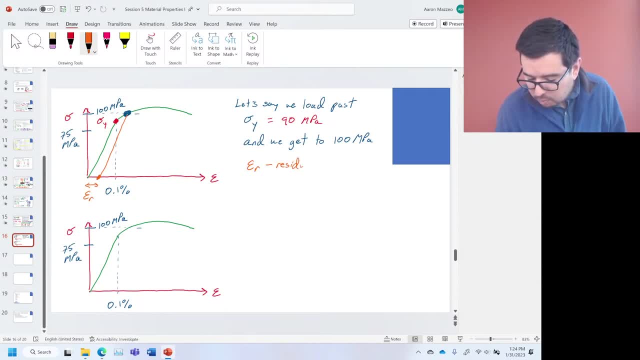 Whoops, Strain. Okay, So you go up beyond the elastic limit, beyond the yield strength, beyond the yield stress, beyond the proportional limit, whatever you want to call it, and then you release the load. You actually come back down with the same slope. 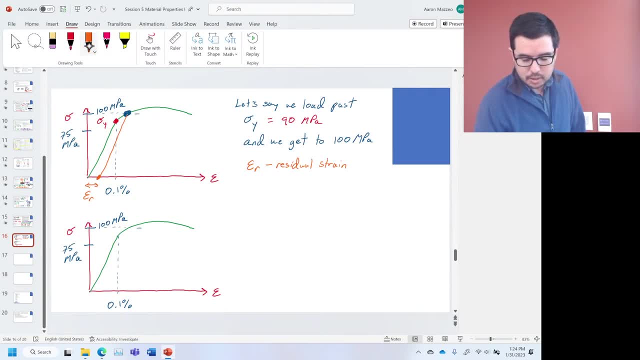 It has the same slope, elastic modulus, Okay, Ah, color: Sure Blue, Right That's. I don't know Whatever, That's not really one. It's not one, All right, It's, But you get the idea right. 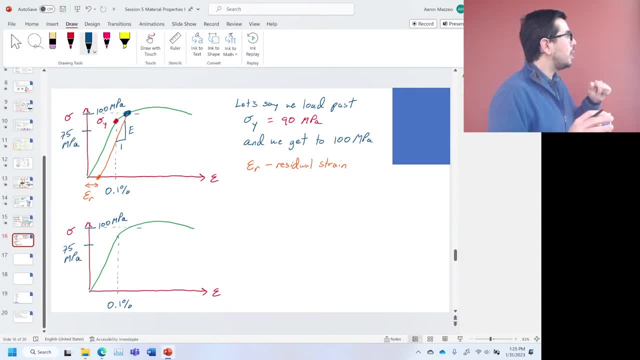 That's going to be the slope. So that is a way to predict how much kind of permanent deformation you've put into your system. Now the other cool thing- Ah, I'm running out of time- The other cool thing is You've actually made the material stronger. 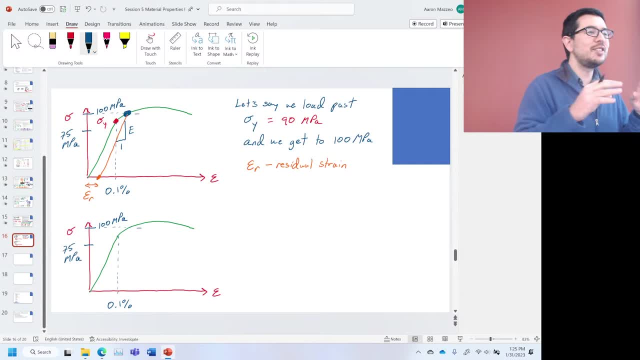 Okay, This is a wild thing. Now I added strain. It came at a cost. All right, It came at a cost, But you've introduced, maybe, some dislocations into the material, if it's a metal alloy, And so guess what? 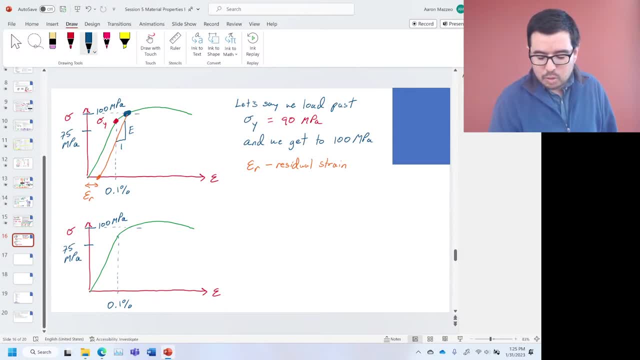 This line becomes the new, This line becomes the new Linear region. Okay, Here, and actually it goes this way as well. Okay To here. Okay, So the material will behave. It will go up and down this new linear region with the same slope it had before. 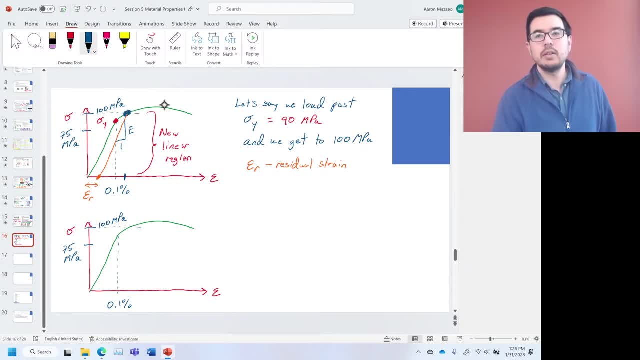 Without yielding Until you get there. Once you get there, it will start to yield again, Okay, So like you could keep doing this, Right, You could keep doing this. You could like come out here And then you'd get a little bit more strain. 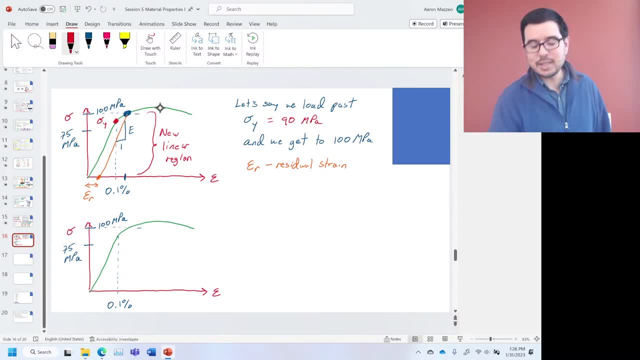 Okay, It has a limit, of course, Because if you go past the ultimate tensile strength, you will have caused a significant change in the cross-sectional area And the material will no longer be getting stronger. Okay, So this is a cool thing with steels. 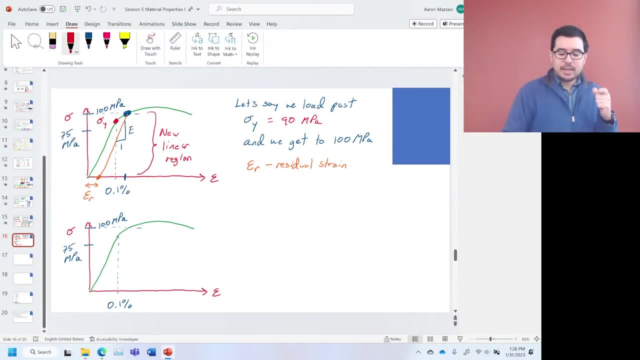 Now Okay. So let's say that you don't know where the yield strength is. Now, let's say we do not know the yield strength. Well, you're given the stress-strain curve. What you do, okay, is you apply this general rule. 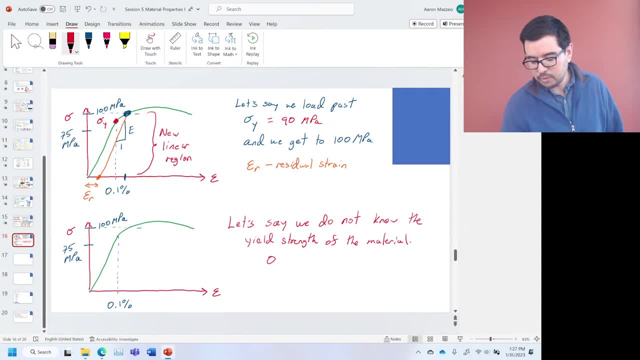 It's called the 0.2% offset rule, Okay, Or method. So we say, oh, 0.2%. Let me pick a different color. Let's do that purple, Okay. So this is 0.1%. 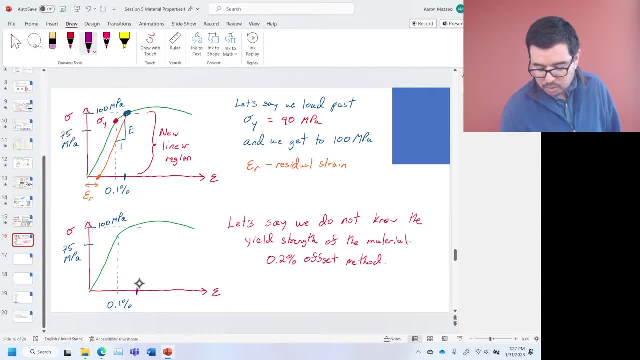 This is exaggerated, But this would be 0.2%. Okay, This one right there. So then, what you do is you draw a line parallel. Okay, This is a bad example, Because it shouldn't go past. All right.